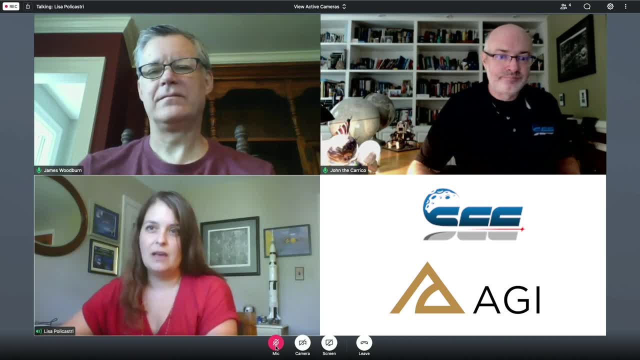 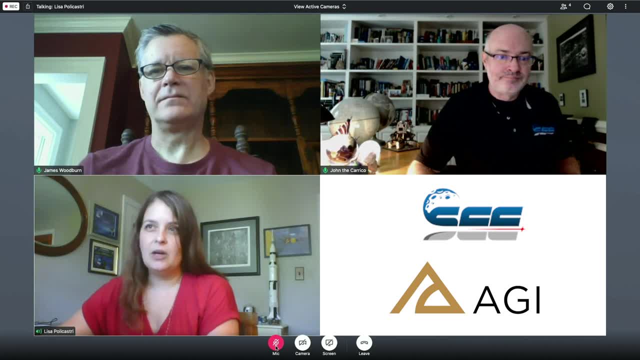 the sixth one, the seventh one, the sixth one, the seventh one, the seventh one, the sixth one, the eighth one, the seventh one, the ninth one and then the last one. So we, you know we were on that mission from the, basically from the beginning, from phase B, all the way. until impact. So about a five-year time span for the mission concept and trying to figure out what it is, you know which tracking ground stations we were going to use, how much tracking data we would need, and then making that into an operational plan and flying it. We worked. 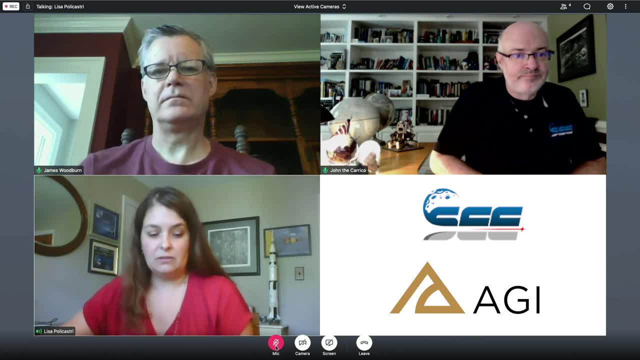 on that mission. It was a big success, I would say. But then the other mission we worked on more recently in 2019, was it Be'er Sheet- when Be'er Sheet Base IL that we supported that mission. The main operators were in Israel, but John and I both worked with those operators. 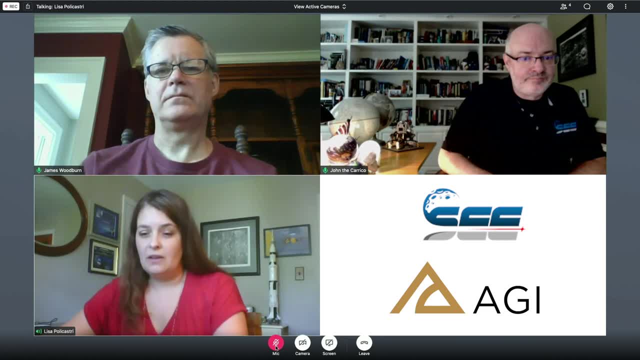 with the flight dynamics team out there. So we were able to do that, So we were able to prepare for the launch and operations from an OD trajectory perspective, And then we helped with flying the mission and going through the tracking data. And, Jim, you looked. 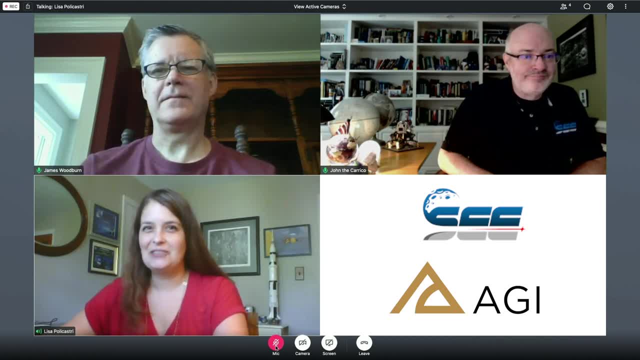 at that data live with us as well, So the three of us all have experience with that. It was a lot of fun that mission, Yeah, and in fact, our videos right now are showing the control rooms where we worked and did that OD. really, if you think about it. 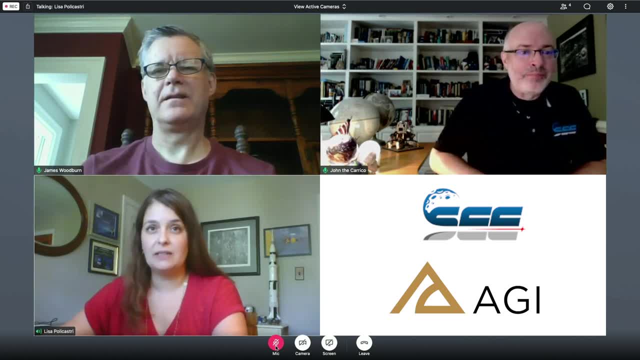 Right, We were remote here in the US while the primary operators were in Israel. Didn't you guys train the Israeli operators as well how to fly that mission? We did. We developed a lot of simulated tracking data, simulation exercises And the team there were very experienced team members for flying. 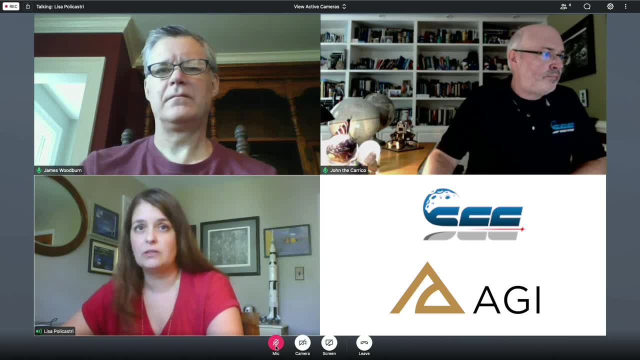 other satellite missions but hadn't flown a lunar mission. So we were able to do that. So we developed some training scenarios and simulated data with imperfect maneuvers leading up to that whole prelaunch timeframe to have that as practice and rehearsals. And that was kind of patterned off of what had been done with LADEE right: Simulating the mission and… Yeah, …the different anomalies and running the flight dynamics team through those types of exercises. Yeah, So yeah, Yeah. 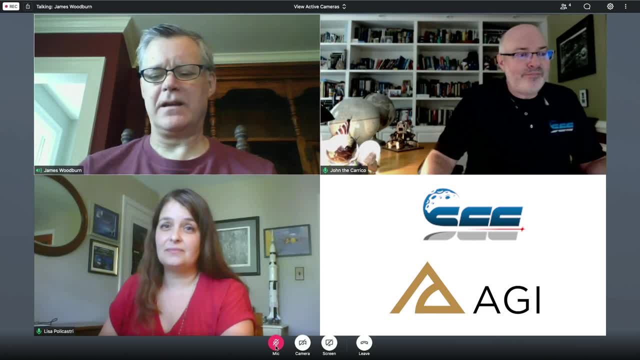 So I think, as you mentioned, the Israeli team was familiar with flying Earth missions, but had not done a lunar mission before. I think that that's something that we're seeing a lot of is that, with the explosion of missions to lunar and cislunar earth missions, 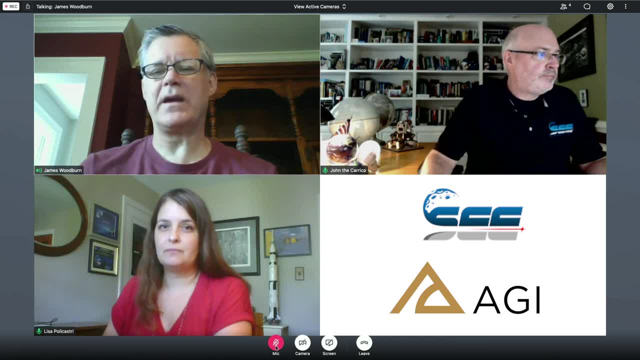 that's going to be a lot faster. Yes, Yeah, this lunar space. there's more and more folks who are interested in flying these types of missions, who have prior experience with flying missions around the earth, but just haven't done missions in those particular regimes before, and so i think one thing that might be interesting to people: 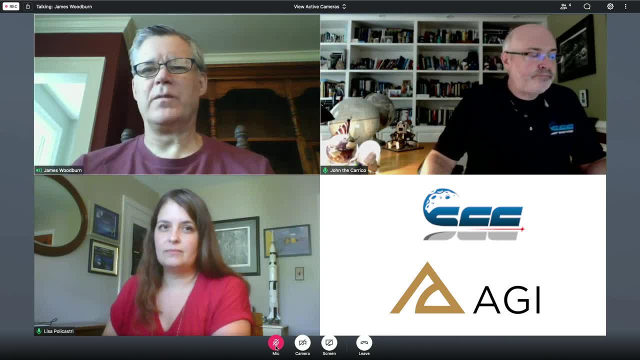 is: how is it different? how do lunar missions differ from earth missions, both in terms of planning and then in terms of actual, you know, flight? i know one thing, john, that you had been talking about earlier was how so many earth missions these days use gps receivers on board. 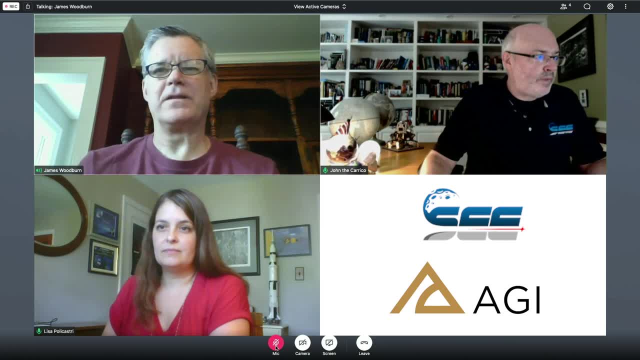 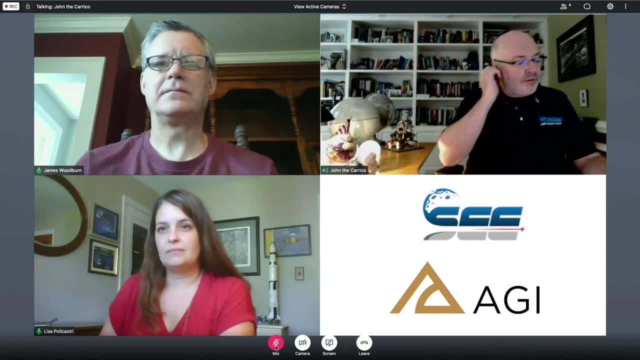 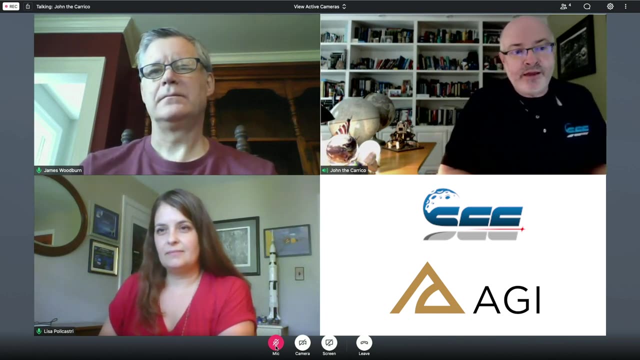 that serves as their main source of tracking data, but of course that's problematic for a mission going to the moon. yeah, that's right. yeah, so there it is exciting. um, it is exciting just to see that there is this big push back to the moon. um, a kind of cool part of it is: 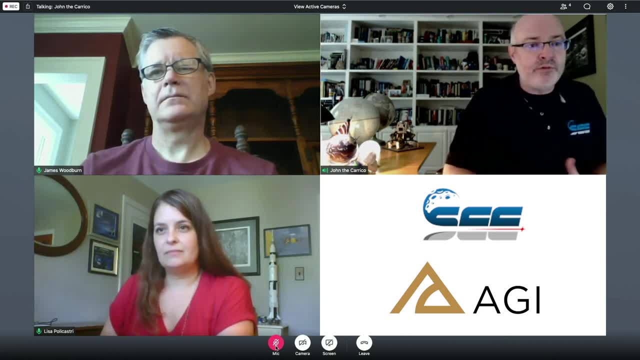 it's not only nasa going back to the moon the way they did in the apollo days, but you've got nasa in the us deciding to buy commercial services to have their payloads delivered. so, like the um nasa eclipse program, the commercial lunar payload services contract. 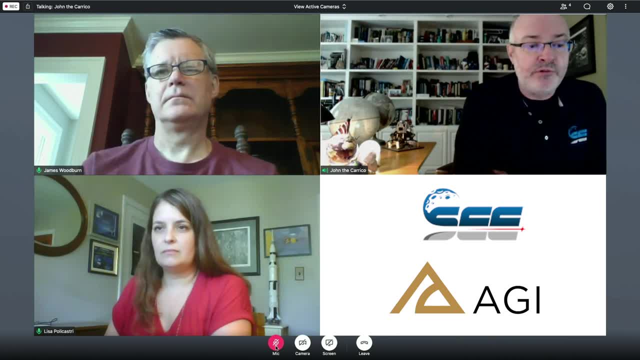 nasa is just buying from commercial companies who are taking these to the moon. so you know, they're building this ecosystem of commercial companies that are a delivery service to the moon. as a result, those commercial companies are trying to hire people who have experience. but because we 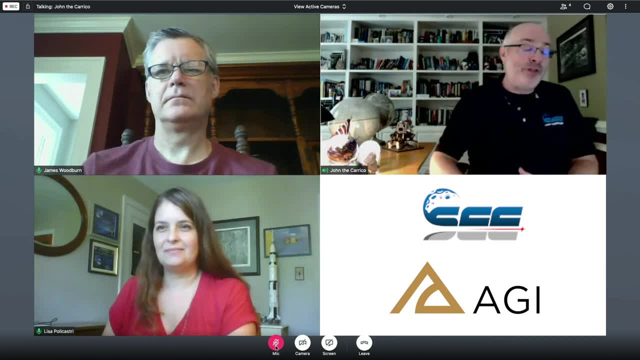 don't have a lot of folks who have flown missions to the moon. what they do is they hire experienced folks who have flown leos and geos, and this is what we saw at space il. they had some extremely experienced satellite operators and they were very good at that, but they haven't seen what the difference is between flying a. 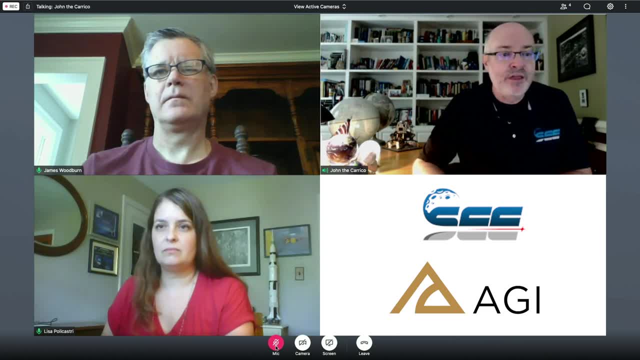 lower orbit or a geo or flying something to the moon, and some of the stuff is very similar and some is very different. but just right now that the need, um, there's this kind of need for people to learn about od and it's too bad we're not doing a webinar on lunar od so people can learn how to do. 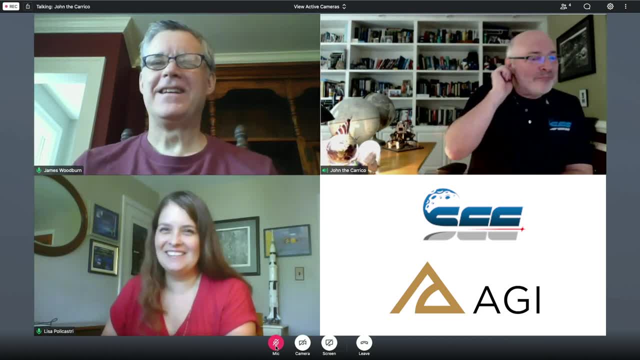 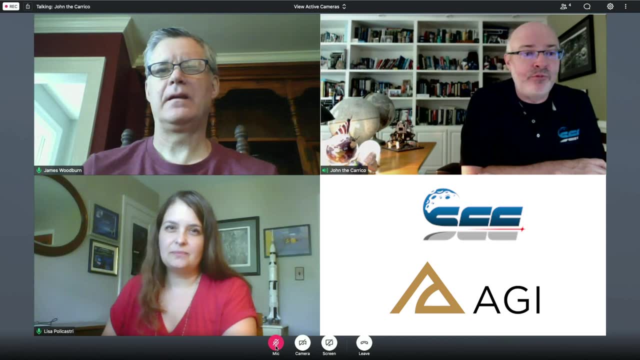 it. it'd be a great idea. that's a great idea. yeah, i think it's kind of funny. i think i t's very funny. you know, what is really funny is a lot of times, Lisa, you and i have run into people who are more experienced than us in flying satellites. 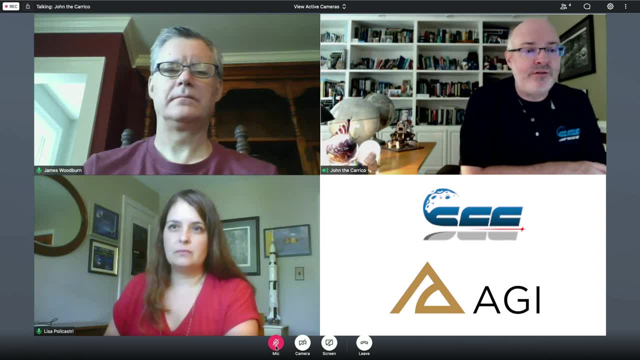 but it's always been around this planet, you know, yeah, so it's been kind of fun to to trade, you know, stories on. well, this is the same as you'd see around the moon, but you know this is different, you know. so back back in the day around the earth people would do radiometric tracking. 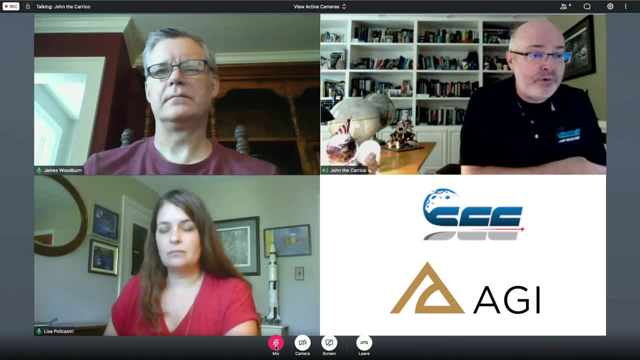 for low earth orbit and for geostationary orbit. we still do range ranging and we use optical angle measurements for geostationary um. but when you get to the moon, there you know you're, you're back completely to radiometric tracking, even if you're a low lunar orbit, there's, there's. 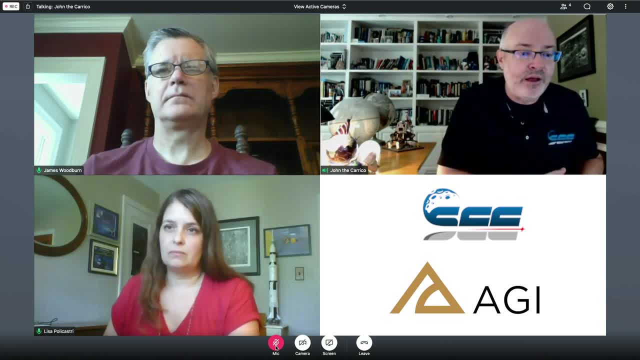 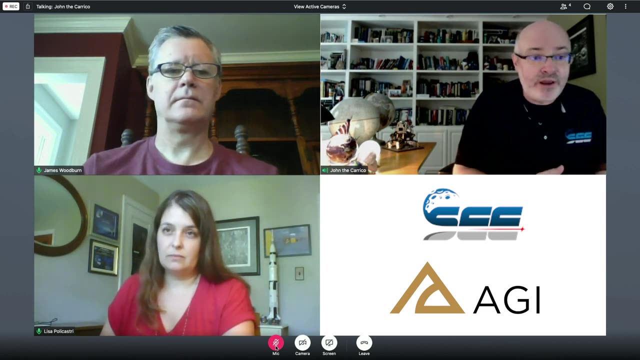 no vps yet. there's some experiments that people are flying that um. hopefully someday we'll have a position, navigation and timing capability at the moon to do, you know, the onboard uh positioning. but right now we're doing, um, we're doing uh, measuring range values, measuring doppler values. 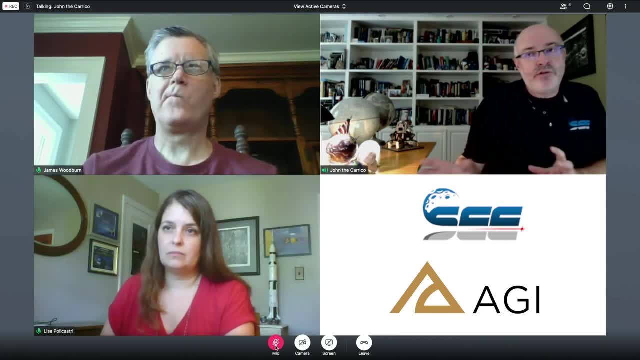 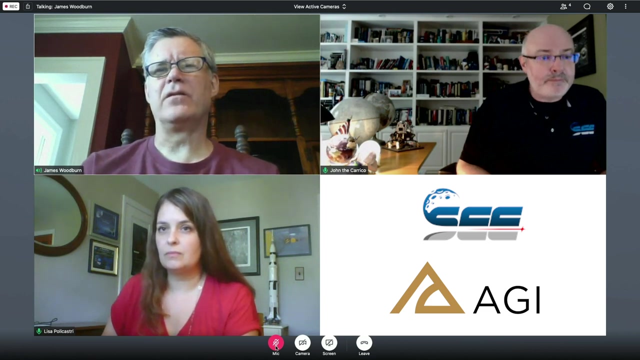 and things like that. so so, so kind of. we're seeing the things that you might see for geostationary transfer or for geostationary orbit, i think you know. am i correct of the, the mmx program? i have that right. is it mmx, the nasa program that had the gps receiver on board? that? used it at really high altitude. yeah, mms, mms, thank you. the mms program um was able to show that you're able to use gps at much higher altitudes. i think that that was some specialized hardware on board. i don't think that was a standard spaceborne gps receiver. 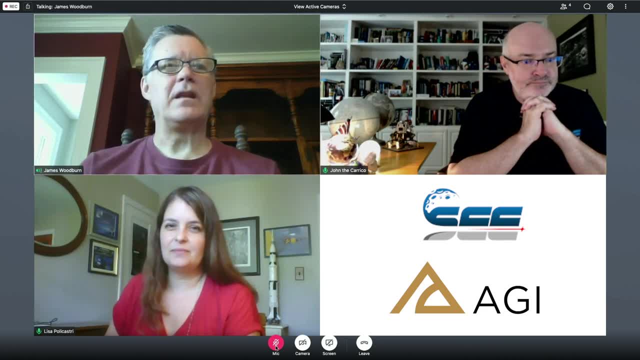 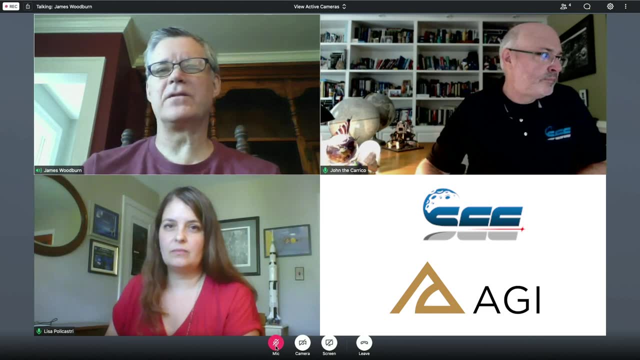 now, with the influx of lunar missions as well, though i think people are also looking at alternative ways of tracking some of the things that we've heard interest in the use of optical navigation technology. um, so we're looking at the use of optical navigation technology, especially during the cislunar part of the mission. 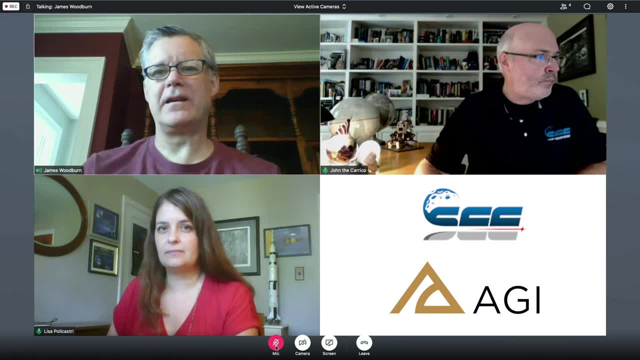 um, people are talking about satellite to satellite tracking, when you're dealing with multiple satellites performing a common mission and we're seeing all different sizes of satellites as well. i mean you used to think of a lunar mission as being a big deal, with a big budget and large spacecraft. 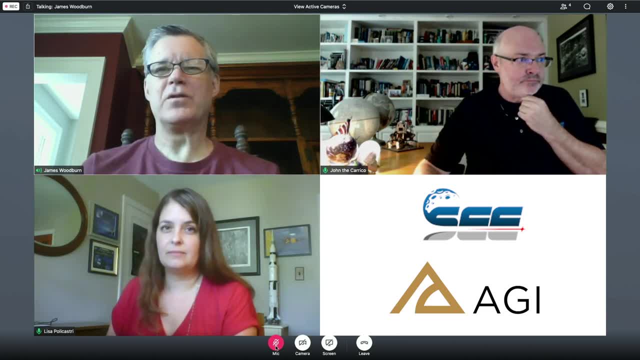 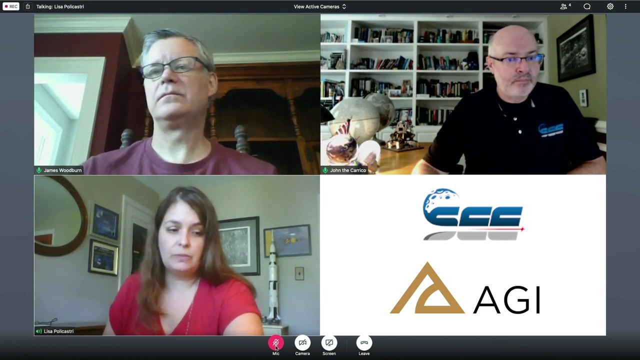 you think back to apollo, you know huge spacecraft, but nowadays we're talking about cubesat missions. right, and what ground architectures are capable of supporting those missions? so with those with the small stats and commercial missions, a lot of them are on the cheap, you know they don't have large budgets, so how do you then they're trying to build the spacecraft. 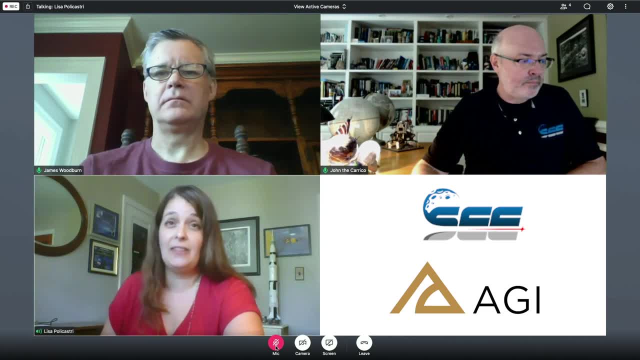 hardware and test that and, you know, pay all the people to do it. and then still, how are we going to fly? it are. how much tracking time do we need to buy from ground stations? what propulsion system are we going to put on this thing and going with some non-traditional alternatives that may be? 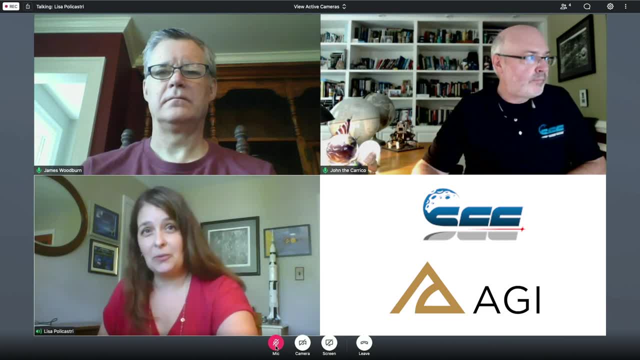 cheaper that area. and then you know, then you're sort of in this infinite loop sometimes of evaluating, you know, all of the trade space of a new propulsion system, while trying to track it and perform critical maneuvers, you know, to capture, until in your orbit it's a lot on the table. 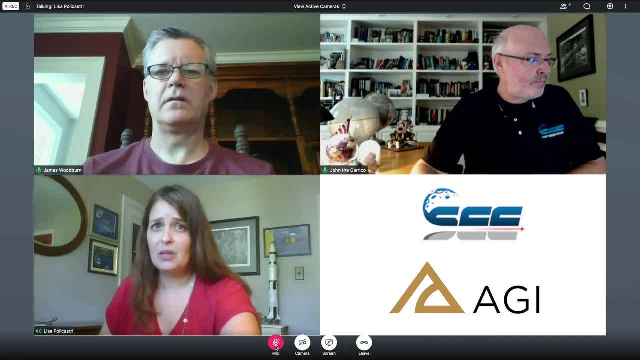 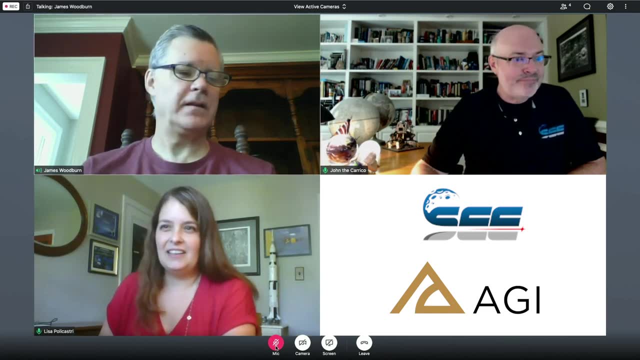 looking at the trade space with these, you know cheaper, modern satellites, right, definitely. and when you think about that, when you think about putting a bunch of new technology up there, like the traditional trajectories to the moon were these, you know, three day, four day, five day direct transfer type trajectories. 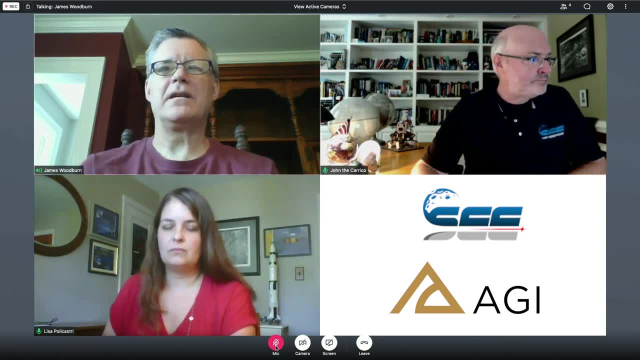 and if you're dealing with new technologies, that doesn't give you a lot of time really to test things out between you know when you launch and when you're going to need to set up and perform a critical lunar orbit insertion. now i know that, um, so some missions apply different types. 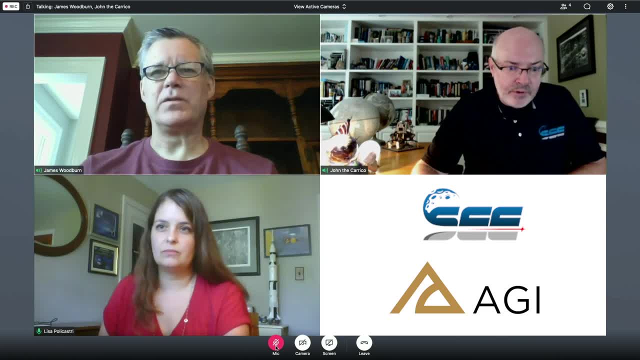 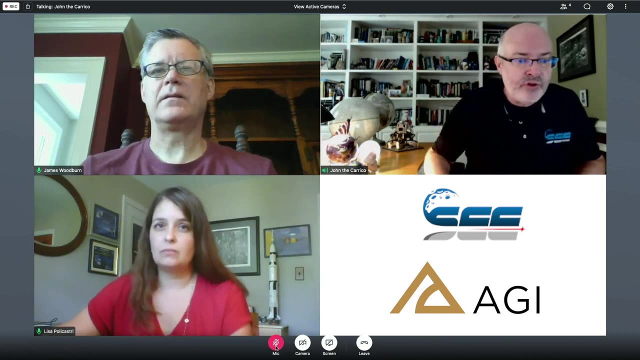 of trajectories to the moon. i'm gonna, um, i'm gonna. i have um, a scenario i can share, um with all the different phasing loops, because i thought we could talk about the different cislunar, because you've mentioned the cislunar transfers a couple times. yeah, 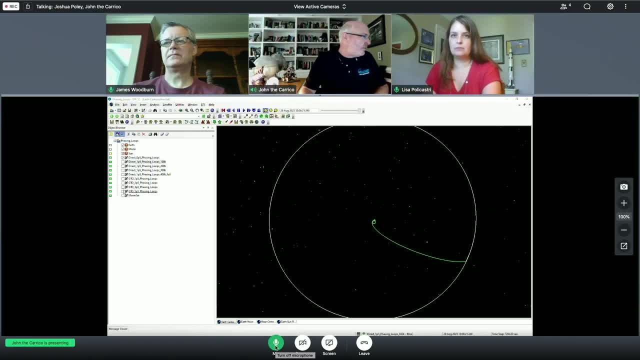 the screen and and and, jim, i can show you that with the apollo, this is the phasing loop. i can show it in this rotating frame where you can see it. yeah, that's a nice view, oh, yeah, so so, um, jim, you had mentioned that. um, you know, the ways that people get to the moon on are different. 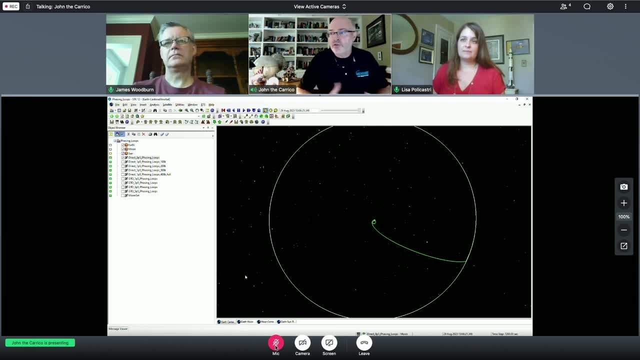 than we've done in the past because of of low cost and because of using ride chairs, getting on different launch vehicles and things like that. so this is an example of a direct five day transfer from here to the moon. uh, this is the moon's orbit in white and this is our home planet, jim, i think. 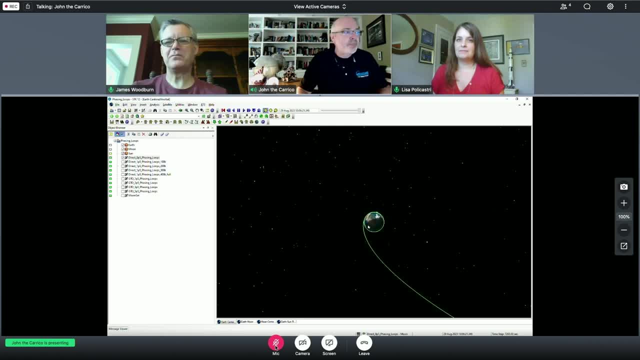 that's where you are right now- were born. i remember right, yeah, yeah, right in that planet. so so that's that's one way to get to the moon, and when you're doing orbit determination on that it's, it's pretty challenging because you never go through a whole orbit right and, as you guys know, like certain, 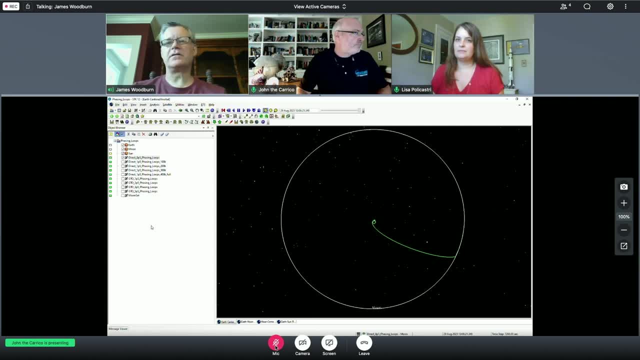 um, things that are estimated along with the orbit, such as tracking station biases and force model parameters. a lot of those don't really become observable on just a portion of an orbit. a lot of times you need one or even multiple orbits for certain things to become fully observable. 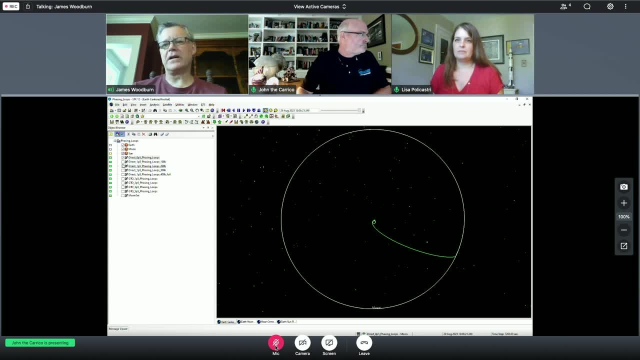 so you know, tracking on a trajectory like what you're showing here, you would be very hesitant to try to use a tracking system that you weren't very familiar with, yeah, one where you need to determine what the biases were in all from the live tracking data. yeah, and so on, um, on, uh, some missions, um. this is an example where we start off in a geostationary. 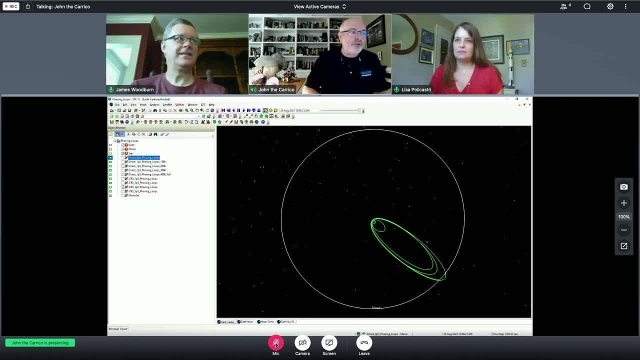 transfer orbit, so um. so this is an example where you might launch on a ride share with a geostationary transfer and then go through a couple phasing groups where you would have some more of these orbits. yeah, that gives you some additional time to figure out unknowns along the way. 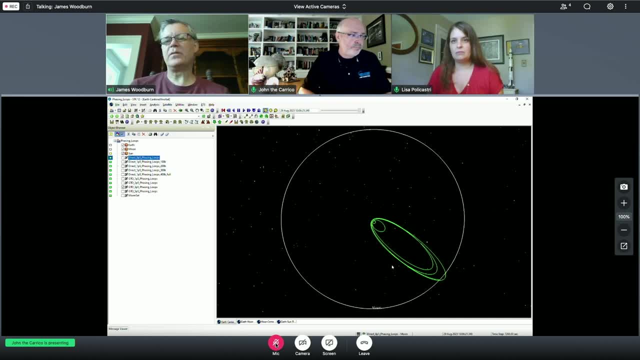 although certain parts of the state may still be difficult to observe, even in these phasing loops, if you have enough uncertainty in your system, it can be difficult to pull things out. so, for example, if you have a number of ground stations that you're unfamiliar with, even with phasing loops like this, it can be challenging to. 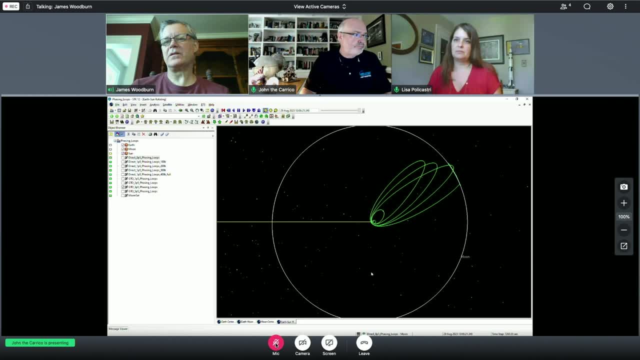 bring everything into step where you want it to. however, if you just have one or two things that are less known and other system or other tracking stations, let's say, that you're more familiar with and you know you can rely on, then you can typically estimate the unknown guys. 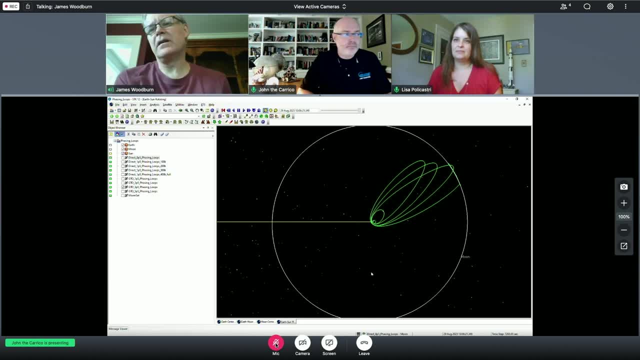 given this kind of a configuration. i think this is also the phasing loops and all i think are also going to be more important with some of the low thrust systems. right, yeah, it's not going to be able to do, you know, the entire orbit change all at once. 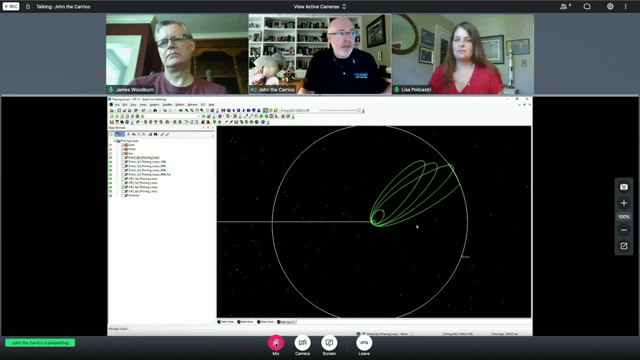 the other thing about the phasing loops, and this is: This is not the Beresheet trajectory, but it's philosophically similar- where we had some geostationary transfer size orbits. then we did maneuvers at Perigee to raise Apogee. 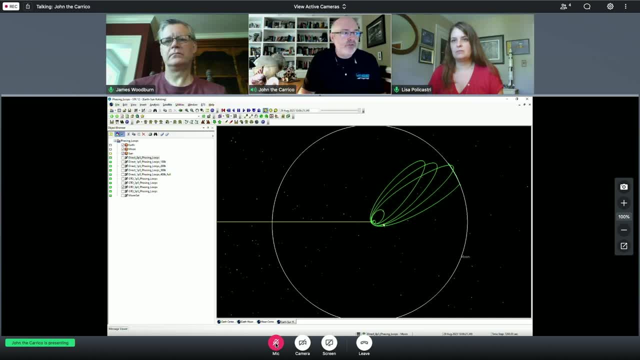 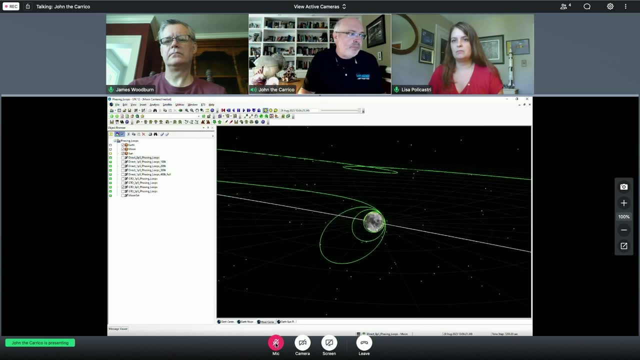 And, as Lisa and Jim, you remember, when we were working on Beresheet we were managing the uncertainty because when we get to the moon we have to perform. really, one of the biggest maneuvers of the entire mission is capturing here at the moon. 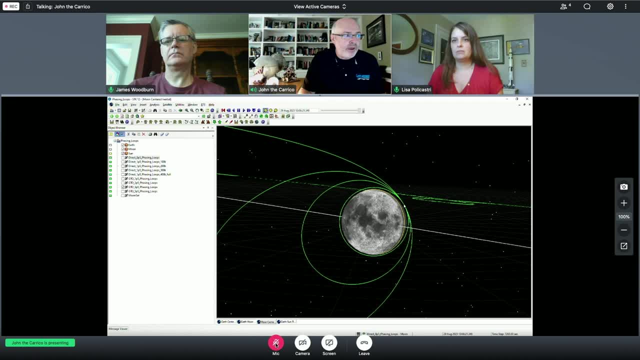 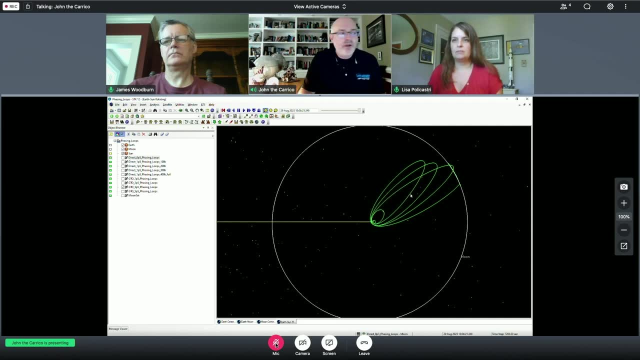 And here we're trying to capture at approximately 100 kilometers off the moon. So I think you guys remember on Beresheet, while we're in the phasing loops, our whole goal here was getting our uncertainty down. So we were within a hundred, you know, we could be within, you know, basically not hit the moon. 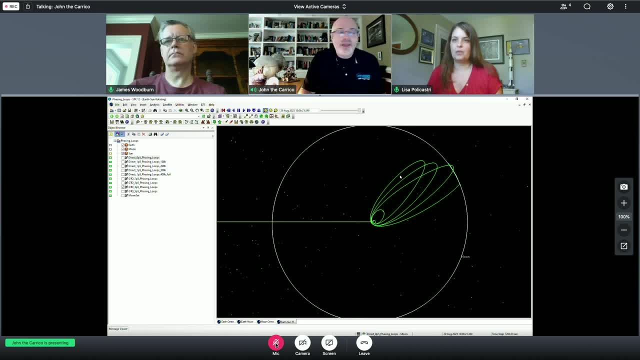 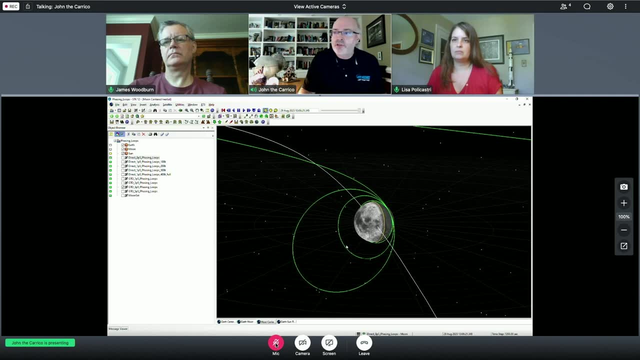 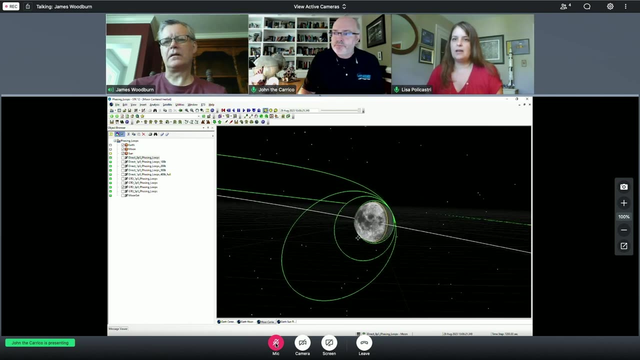 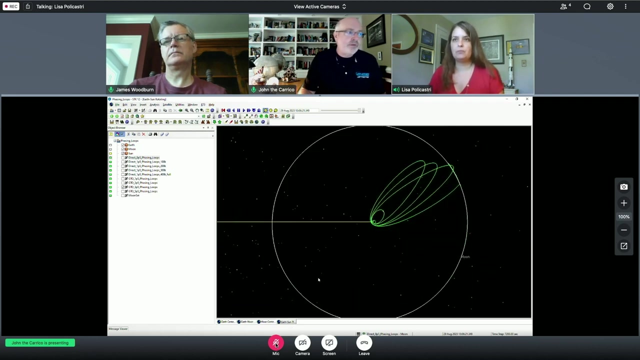 We want to be 100 kilometers or greater above the moon. And now this phase of the orbit determination is a lot different than once you capture around the moon. It's almost like two different missions from an orbit determination point of view. The timeline that you were just showing, John, was about a month from launch to lunar capture, right? That's right. Yeah, That's how that's different. Instead of it taking, you know, five days on the direct transfer, it takes about a month to perform multiple maneuvers, But in the meantime you have time to test out, you know, or evaluate your engine. 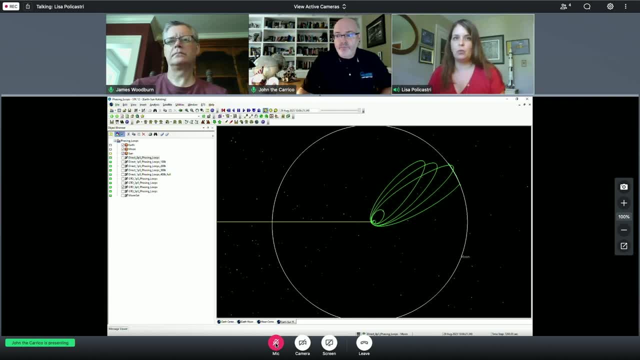 What's the performance we're getting out of the thrusters? What are the- you know- tracking, calibration activities you're doing between the transponder versus the ground stations? And you might have a little more time to look at all of that and have time to work out any kinks you may have on your- you know your- new spacecraft before you get to the moon. So you have that month long timeframe. It's not relaxing because you're still doing multiple burns and planning and your next maneuver and reconstructing the previous maneuver, all to get to the goal of capturing the moon. It's not a relaxing one month, but it is. you do have more time to from a spacecraft, from a system point of view. 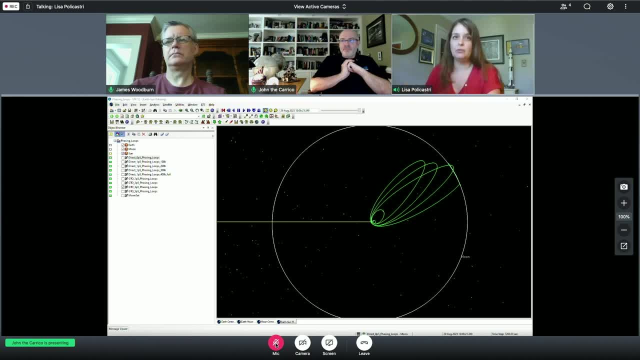 to work out any unknowns, or at least try to. Yeah Lisa, I think that's probably one of the unsung heroes of orbit determination. You know, when people think of orbit determination often they think, oh well, where was the satellite? 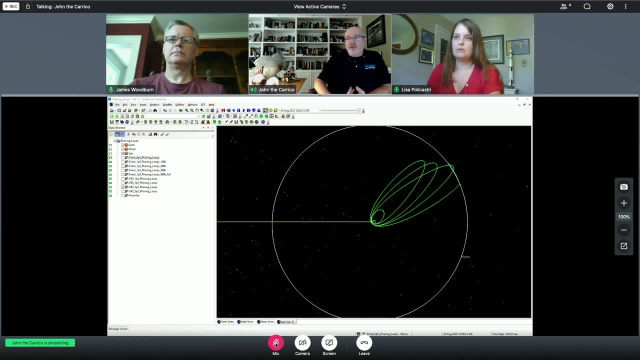 But really an important part, like you said, is, you know, calibrating the tracking system Because, Jim, like you mentioned a lot of times, with these commercial companies, it's the first time they flew it. And then, Lisa, you mentioned calibrating the engine. 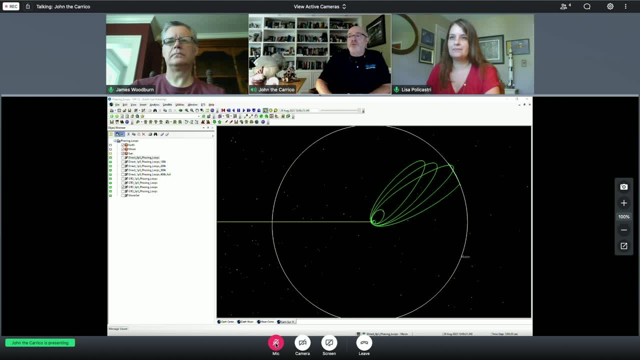 It's the first time. Sometimes it's the first time that engine's even been built. It's never been used before And you have to do like a 600 meter per second or more maneuver to capture in at the- you know, at the moon. 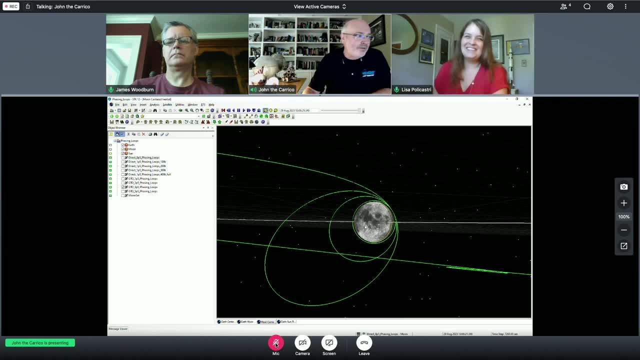 You can break it up into different ratios. Some of them have to equal 800 meters per second. So you're getting ready to do this big engine and you've never fired it before. So if you go on this direct transfer, the first time you fire the engine. 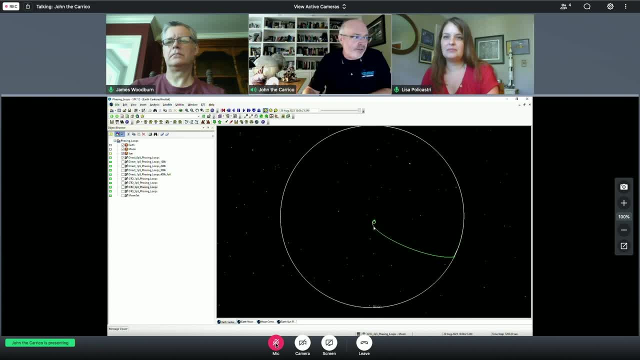 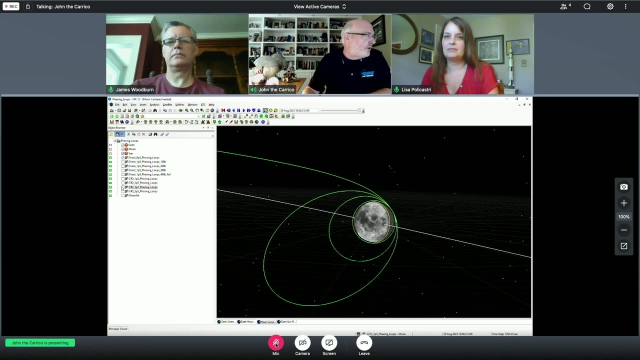 so if you go on the direct transfer and you're thrown on this trajectory the first time, except for maybe a small couple meter per second trajectory correction maneuver you would fire the engine is right here And it's not calibrated at all, Whereas if we go on these multicast. 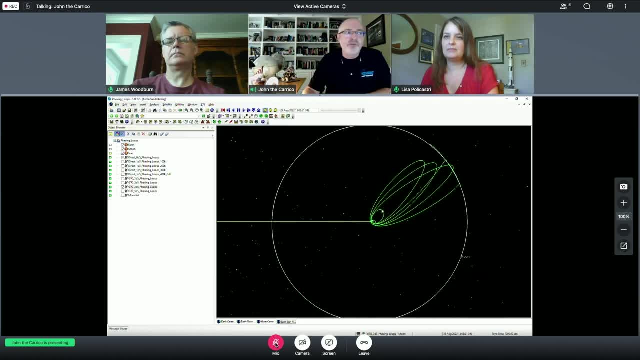 the phasing loop trajectories. you have many maneuvers where you can calibrate the engine And I don't know, You know some people might not think of orbit determination as calibrating your hardware. That's what I was just going to say, or reiterate again. is that you know? 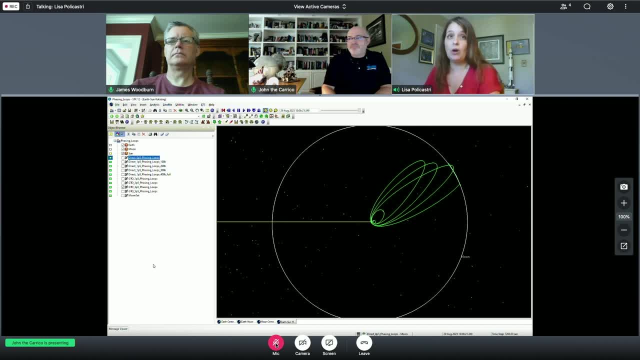 traditionally we think of orbit determination as like an estimate of where we were, where the satellite was. It's important for a lot of reasons, But really too, you're taking your last state from your last measurement and you can apply your uncertainty and propagate that forward to help plan your next event. 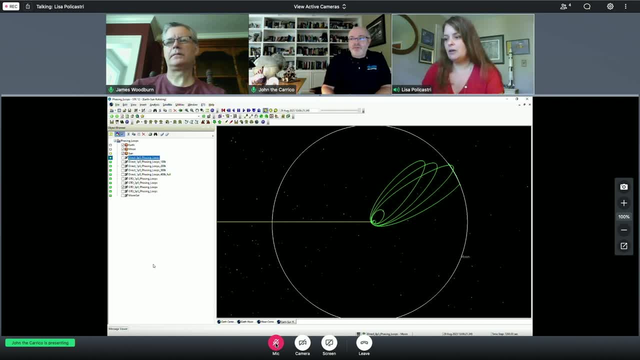 The other thing is: you know when we're doing orbit estimation, where we were. you know a lot of times it's important. for once, you're performing like a science mission, you know. so you've got your. you're already around the moon. 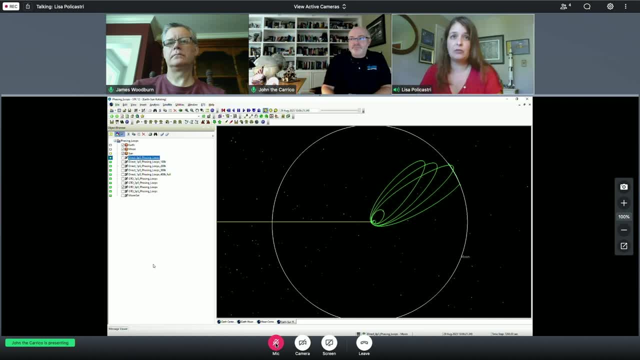 you have your payloads that are performing, or your instruments that are performing, scientific measurements or scientific activities, And a lot of times the scientists want to know where were we around the moon when that, when those measurements or those collections took place, so that they can do some correlation with their data. 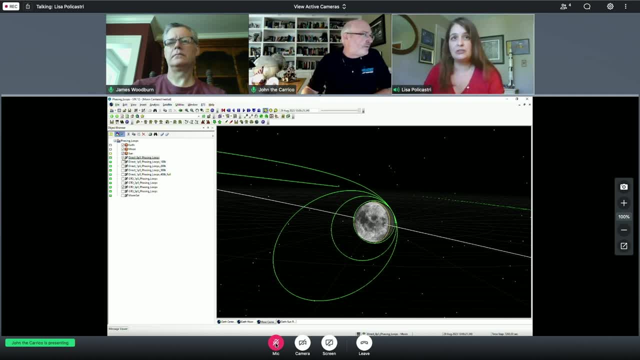 But so that's really important too is the post-processing of all of the tracking data to deliver to the scientists. so they know, oh, we were coming right around, you know the lunar horizon, or we were coming right around, you know, over these specific areas of the moon that they were interested in collecting data on. 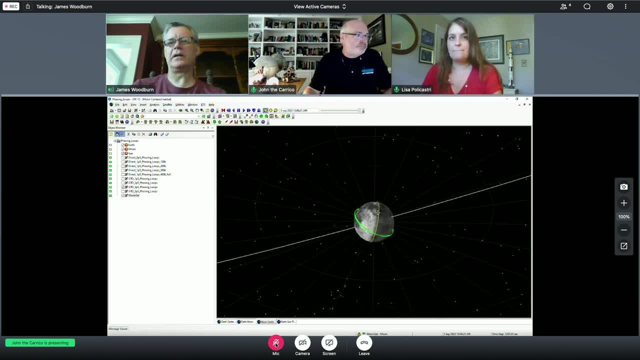 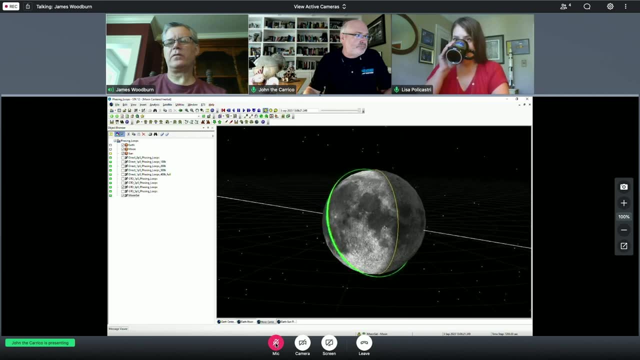 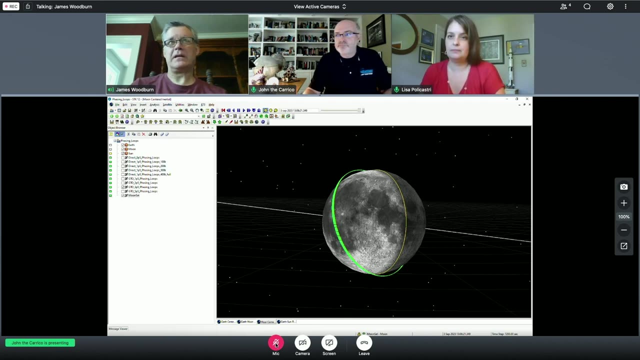 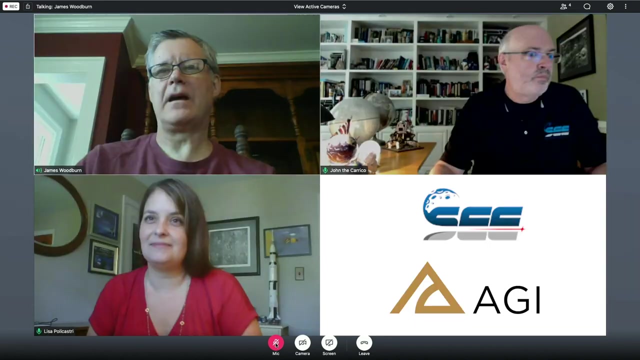 Lisa, you mentioned about, you know, calibrating the engines, And when you're performing these maneuvers in the phasing loops, you have to remember as well that it takes a little while to for the orbit determination process to hone in on how that maneuver performed. 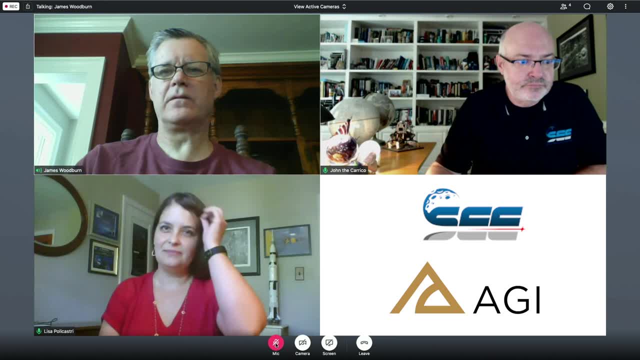 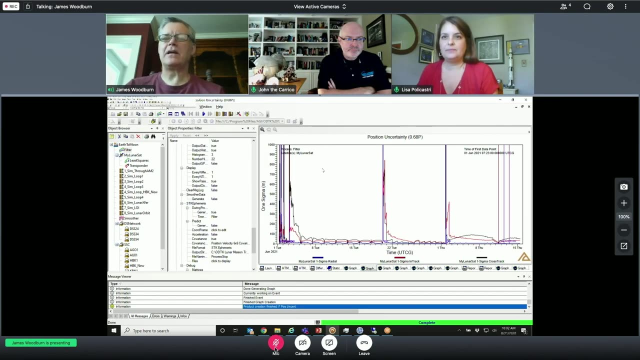 And John, if I can share my screen, I can show you A little bit of an example of OD, based on a configuration very similar to what you were just showing. OK, so what this is? this is an uncertainty plot coming off of a filter that's operating on simulated data. 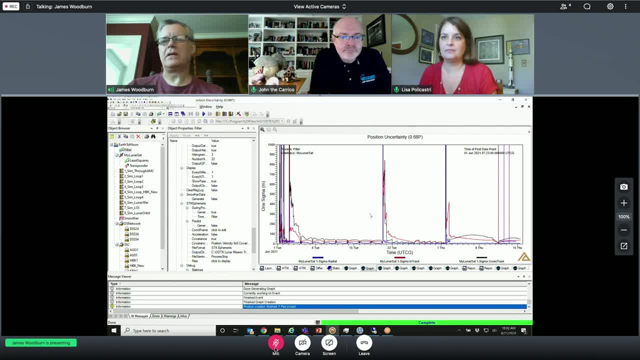 but is operating on a scenario very similar to what John was just showing, where you have multiple phasing loops on your way out to LOI at the moon, And these purple lines here are representing where the maneuvers are in this scenario, And then the blue, red and black lines are representing the trajectory- uncertainty. 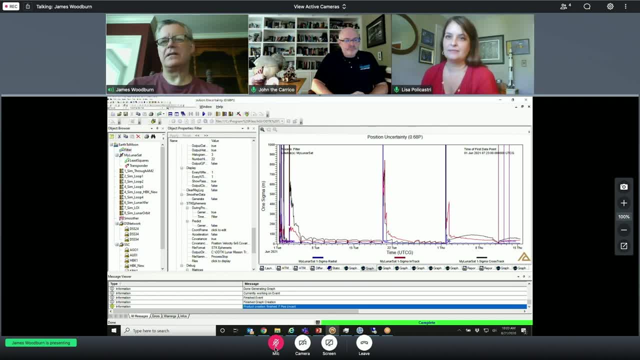 in the filtered estimate. So at each maneuver, what you see is that the uncertainty in the filtered estimate jumps up and then it comes back down as we receive more tracking data after the maneuver, And this is representative of the fact that maneuvers have a lot more inherent uncertainty. 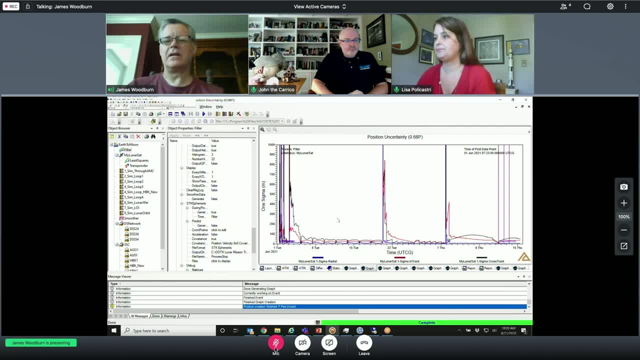 in the forces that they're applying to the spacecraft than the forces from the natural environment. So, when we take that into account, the uncertainty in the spacecraft position and velocity increases over the maneuver. So what you can see, though, is that it takes. 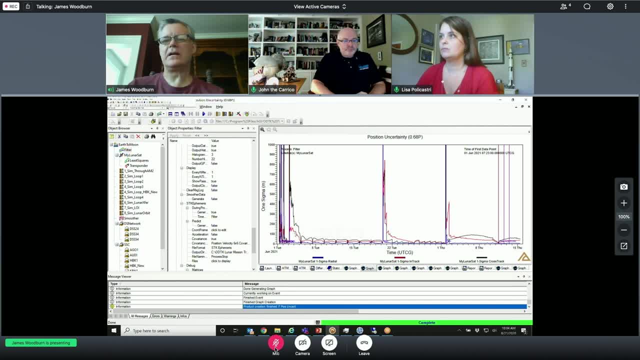 even after you start tracking on the other side of the maneuver it can take a little bit of time for that maneuver estimate. I'm sorry for the trajectory estimate to get back down to kind of a nominal level of uncertainty And you know we're looking at, for example, on this maneuver. 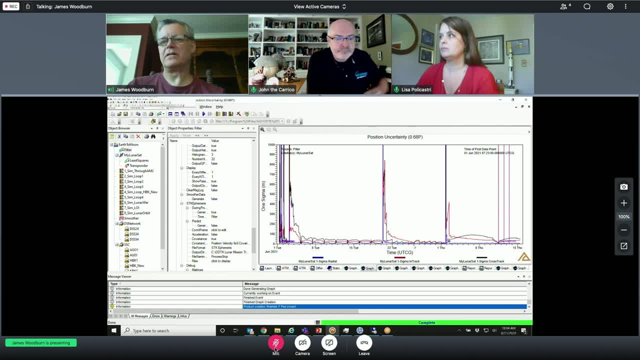 we're looking at a number of days, each one of these tick mark spheres a day. We're looking at a number of days before your complete uncertainty gets back down to a nominal range. Now, these orbits themselves are on the order of a week or so. 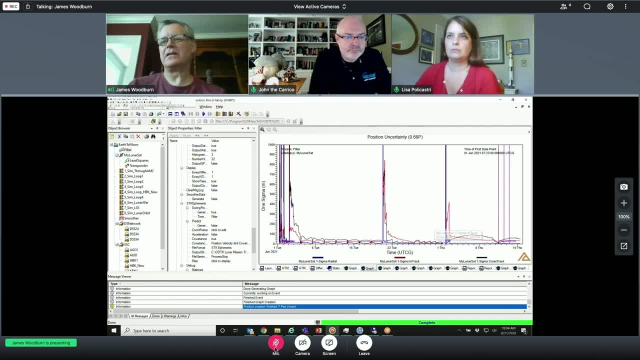 So it's still. you know you're recovering accuracy in time to do your next maneuver, But it does take some amount of time to regain the accuracy, And this is also representative of the amount of time it would take to figure out how the engines are performing. 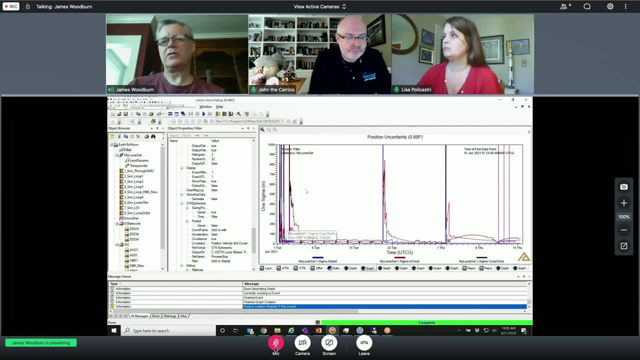 So as we move along here at this end we're on the smaller phasing loops, And then as we move to the right, we get on larger and larger phasing loops And you can kind of see how the amount of time for accuracy recovery keeps stretching out. 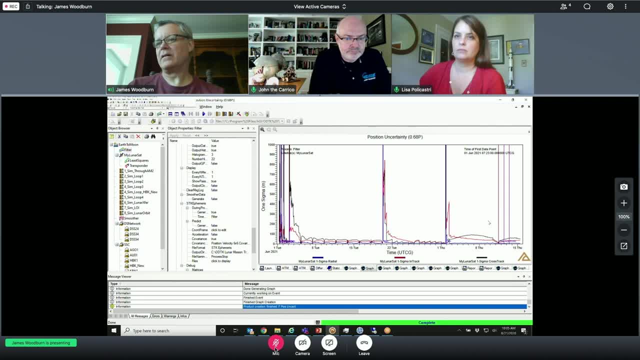 So it is related to the orbital process And you can see how long it takes you to recover. And then, if we look over here, this is actually a graph of the LOI maneuver. So we have LOI here in the center-ish of the graph. 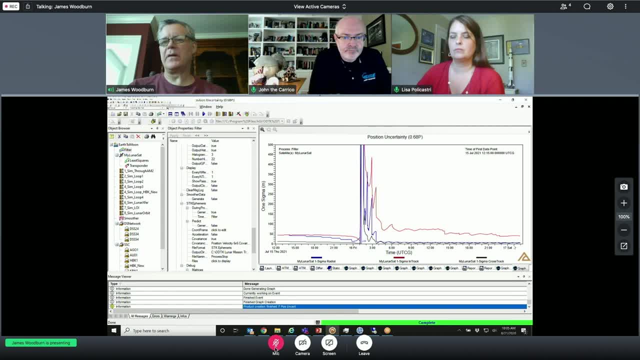 And this is a much smaller time scale. now We're showing only about a day and a half total time on this graph And you can see that the uncertainty of course jumps way up going across LOI. But now remember that after we've gone through LOI, now we're in orbit about the moon. 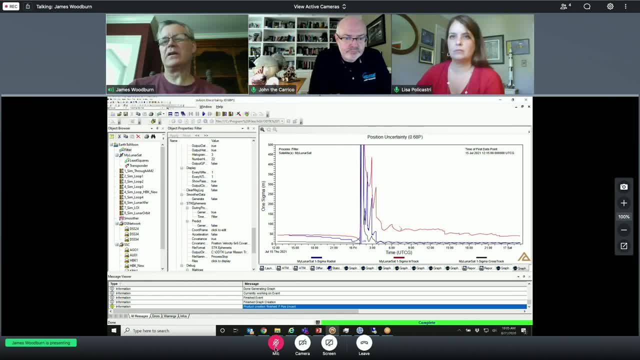 So when we're in orbit about the moon, and in this case we're going into a lower orbit than what John was showing, This is going into a 400-kilometer circular orbit of the moon, But now our time scales are driven by the period of the lunar orbit. So we're now not taking days or weeks to recover to a nominal accuracy level Now. we're mostly recovered in a matter of- well, I would say- six hours-ish here. So in that sense you know, it's taking us a couple of revolutions around the moon to recover. 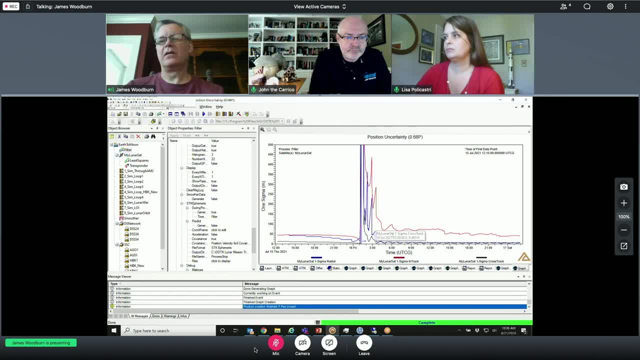 But it's a much shorter time scale because of the fact that the orbital period is much shorter once we go through LOI. So one of the things that this analysis is used for is to figure out how accurate it takes for you to recover from the first lunar orbit insertion. 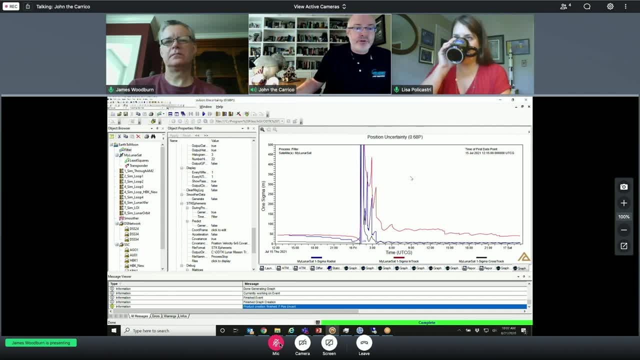 And then how many revs before you plan the second lunar orbit insertion? If your uncertainty is still too much, you won't even be able to plan it, let alone calibrate the engine. And that lunar orbit insertion one is where you on some spacecraft. 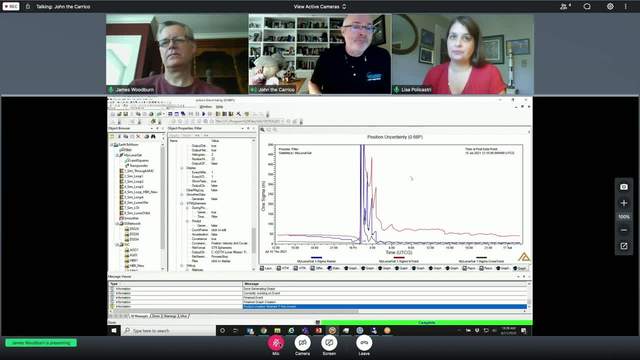 is losing like half the mass of your spacecraft in propellant. So you've probably heard me say this way too many times, but I always think that flight dynamics and orbit determination is like Rodney Dangerfield, that you get no respect. But a lot of times when a mission planner just says: oh well, you know, we're going to be really, you know, sporty and we're going to capture and we're going to do three maneuvers- 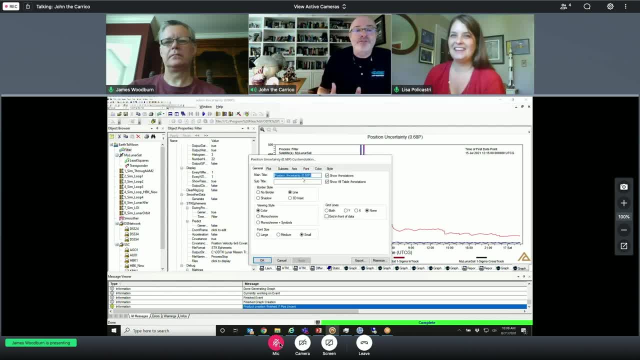 And then we're going to go into orbiter land. What I think you're forgetting is: well, don't forget about orbit determination. Can you really track it? Can you calibrate your engine? You know, this is a brand new spacecraft and you're far away from Earth. 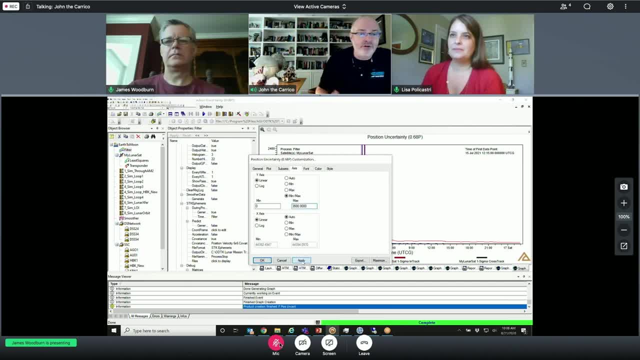 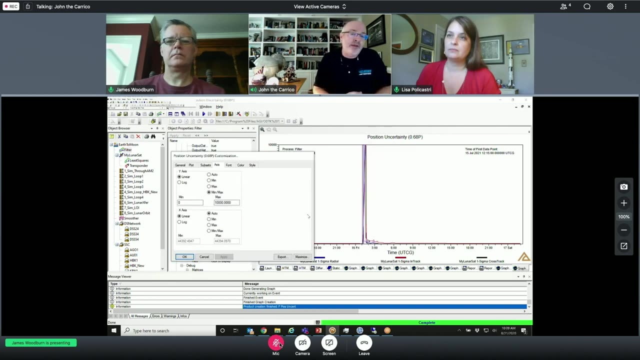 So I think doing these analyses early in the mission planning really helps understand. should you buy a better radio? Should you buy more time on the ground stations? You know what You know if you really have a time. Does the orbit determination support? 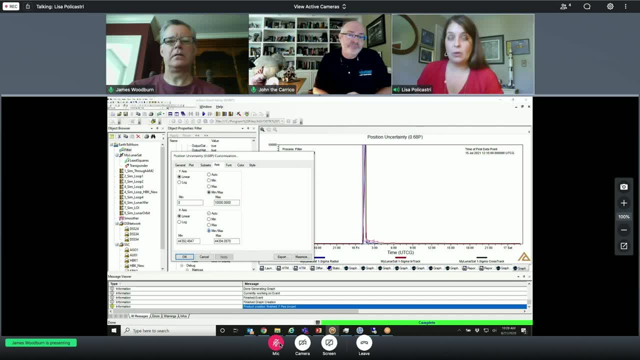 Yeah, oftentimes, when missions are proposed, these type of things John just mentioned aren't thought of yet You know, building an initial mission concept and focusing on what the mission is going to do, without necessarily paying a lot of attention to detail how you're going to get from here to there. 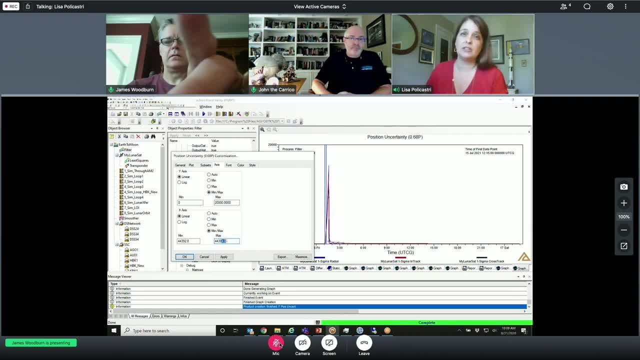 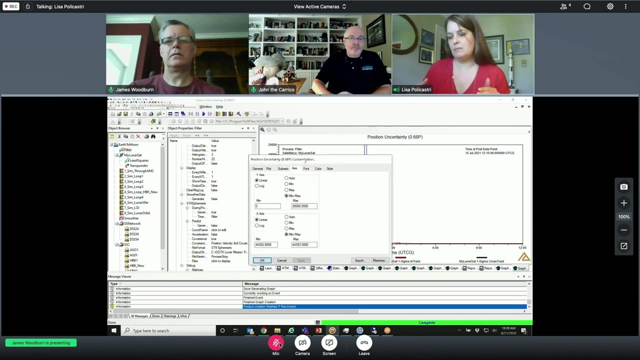 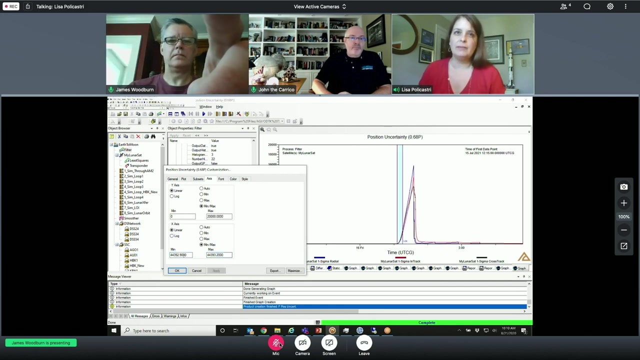 And that's where orbit determination comes in. Orbit determination error analysis can be really helpful to have information about the mission timeline And you may end up having to get a whole different trajectory or design a whole different trajectory because you didn't consider all of these operational timeline things that you have to do. 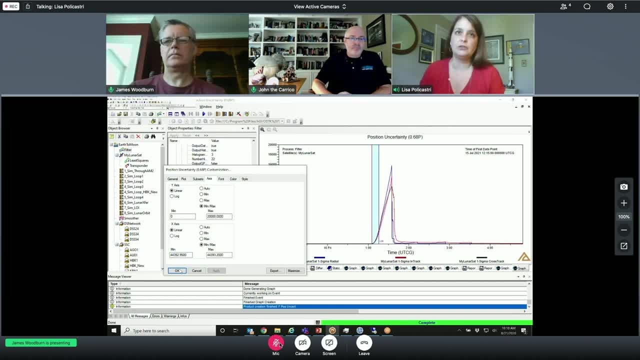 And you know, OD error analysis. you know, using the simulated data, just like Jim was describing- can really provide a lot of insight into the whole mission design When you're deciding, in the end, which of these trajectories do we want to take. 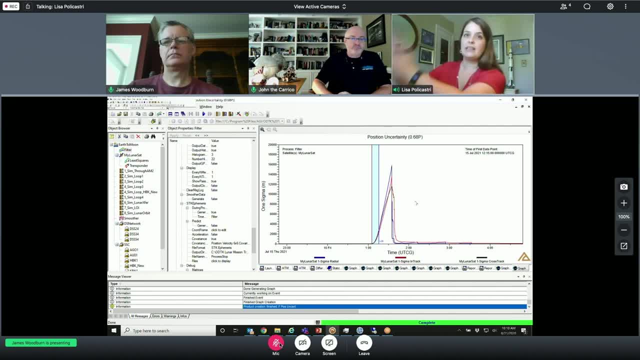 And you know, a lot of times folks may say, oh, we just want to get to the moon, We want to get there fast, We don't want to spend a lot of time in there, We want to get to the radiation belt. 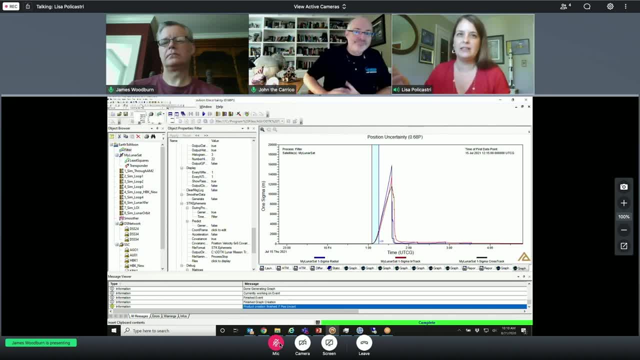 Or you know it's a new spacecraft. You know we want to get there fast and get there, because the longer you're in orbit, the more things can go wrong, You know. so it's not trying to say people that think that way are wrong. 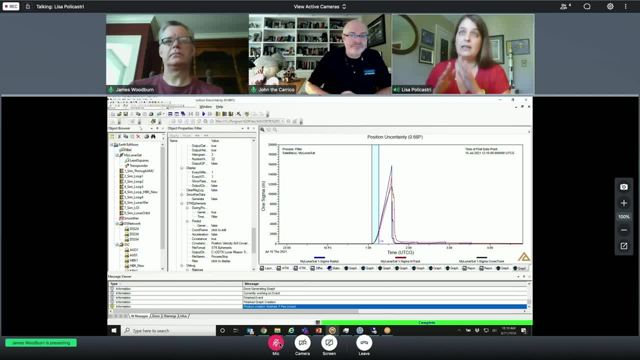 It's just, that's one way to think about it, But it's an incomplete picture, Yeah. And then when you do the OD simulation, With a variety of tracking schedules, with uncertainty in maneuver performance, And when you look at it all in a big picture, you have a well more informed mission design. you know that, okay, this is a flyable trajectory, even though we may not like it as much as our earlier design. 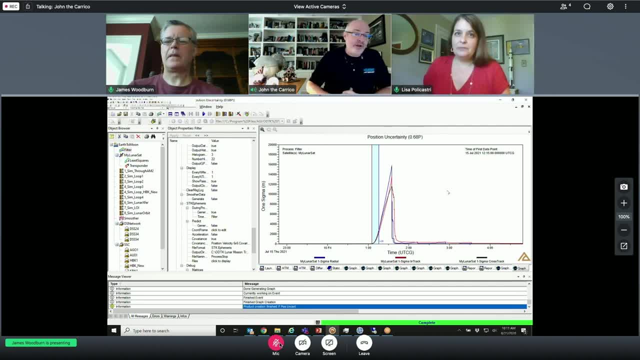 Yep. Well, the other thing is ground station availability. You know, if you're used to flying geostationary satellites, Then you can always see your satellite from your ground station Whenever you want to see it. you know, if you're flying in lower Thor of it, you don't have to worry about tracking. whenever you can talk to a ground station- and they can be small dishes that you can talk with- 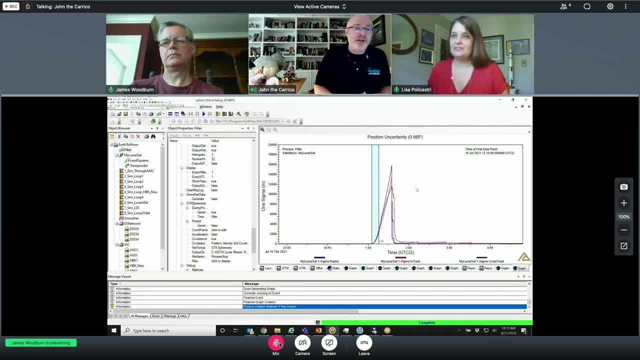 You can tell them either the GPS data down, But here you have to coordinate with ground stations And if you're at the moon or on the way to the moon, You're really can only track the satellite when you can see the satellite And then you can see the moon. 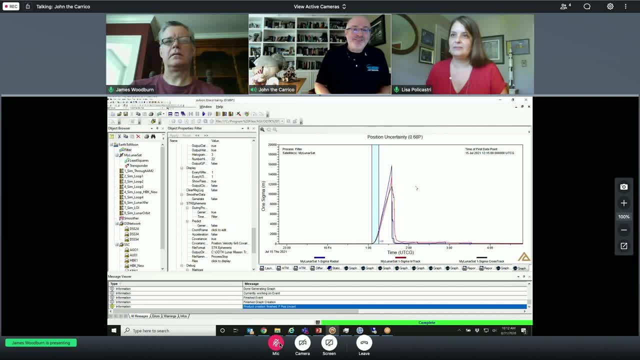 And so that's, you know, not even half the day. So, um, I wanted to put a plug in for this movie, the dish Sam Neill and Patrick Warburton. everything you need to know about tracking lunar satellites is done in a very family friendly way in this movie. 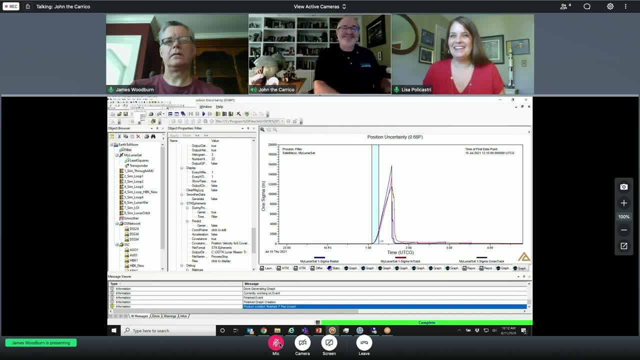 I get very little money for promoting this, but So, anyway, definitely go and see the dish, But but it really is. I think that we see, you're right, when people think about mission planning, They think, oh, we have consumables, we. we can only spend five days to get there because we're going to boil off the propellant or, like you said, radiation. 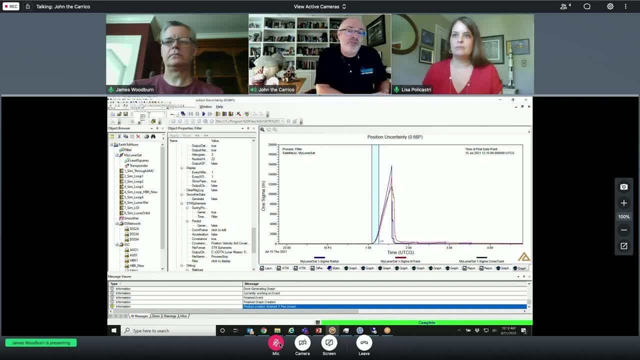 Those are all hardware decision, but so is your ground station and your transponder. Those are hardware decisions, Right, And can you track it? can you actually? is your engine that you're specifying? Is it accurate enough that you can do lose orbit determination, or are you using something that is so brand new in your engine that you need to do tight orbit determination and more tracking so that you can calibrate? 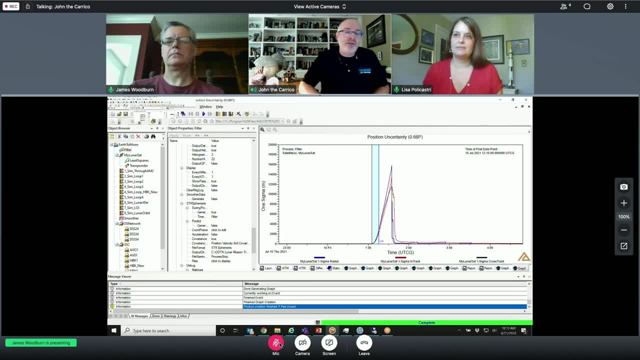 And there's a huge trade off that we said I don't think we've seen very done very often, like the pre phase eight parts of the studies or the early studies. Yeah, a lot of times, Yeah, Yeah, Yeah, we've seen these decisions that we've seen, as you know, reviewers or even participants, and when we get brought in at some point after our mission is awarded. 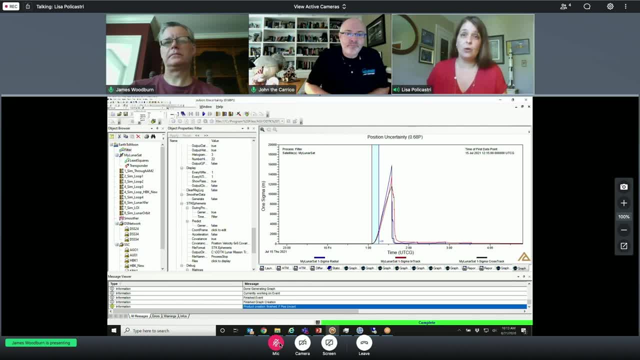 You know, when we look at the onset Like it is, like you were saying, eight, the concept is based on always a subset of the hardware decisions that have not taken into account, like a full OD error analysis. and when I say full od error analysis, 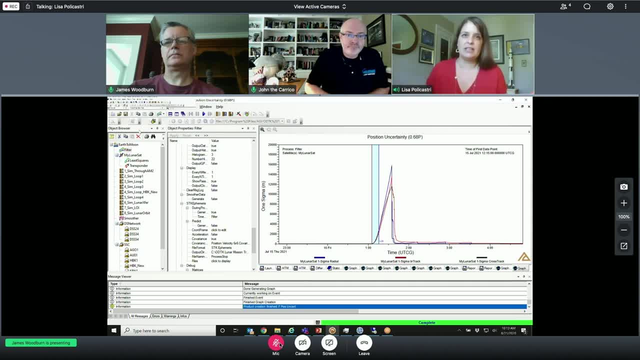 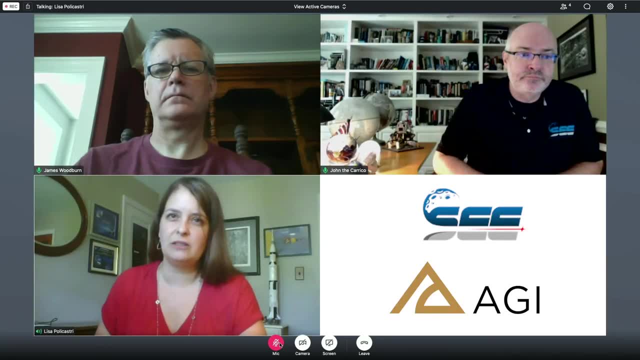 It's just like a feasibility, like something that's representative, that's really just doing that sort of a once through when you're developing your early mission feasibility concepts and that kind of work. you know, having that as a part of the design is more complete design. 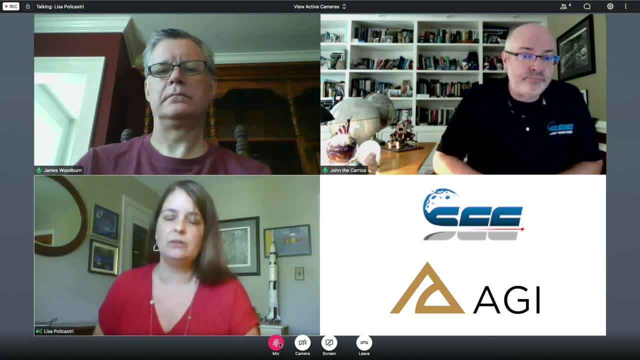 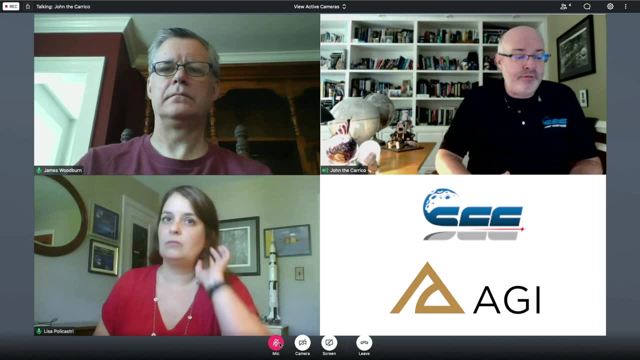 Yeah, do all kinds of cases. later on, you know you can look at all. Yeah. Yeah, We didn't just even described, I mean, if, if there's some people watching this that haven't done or haven't heard of orbit determination, error analysis, it's kind of, Jim, what you just did. 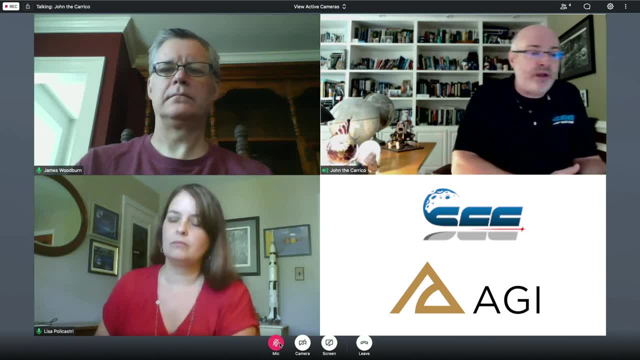 You come up with a candidate tracking hardware, candidate ground station, candidate tracking schedule. You know we simulate the observations And then make pretend those are real observations. We then do orbit determination and see can we calibrate that engine. Maybe we have enough tracking data. or how many revs after the maneuver goes off. 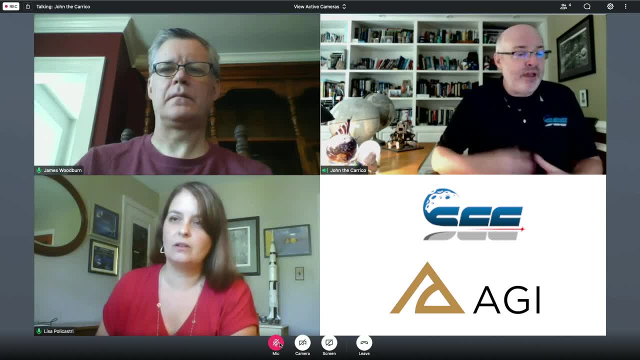 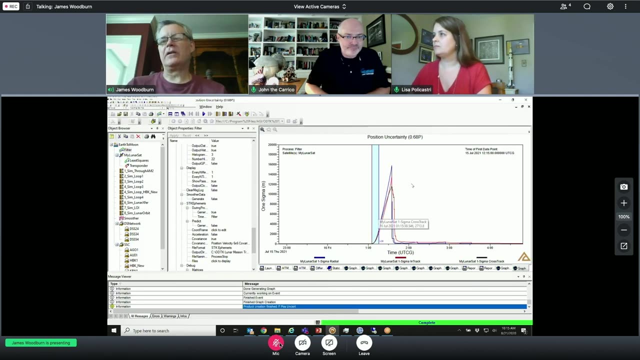 Before we're ready to plan the next maneuver. it's, it's. it's not some hard optimization thing, it's just: Oh right, get one pass today. what if I get two passes? Yes, What if I get a tour So you can see some things like at the LOA here? 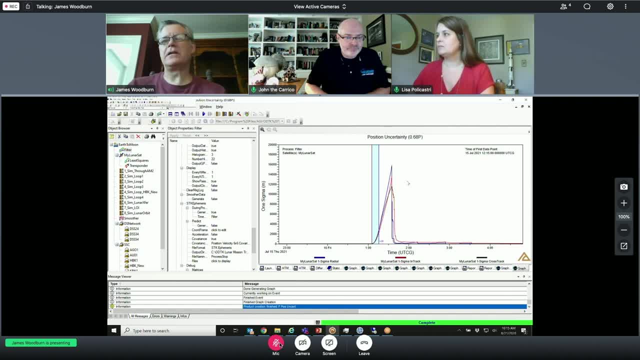 When you guys were talking about the need to schedule the ground stations and all that kind of stuff of stuff and how important it is to have a ground station contact very shortly after the llr. i've zoomed out on the loi a little bit so that we can see the full growth of 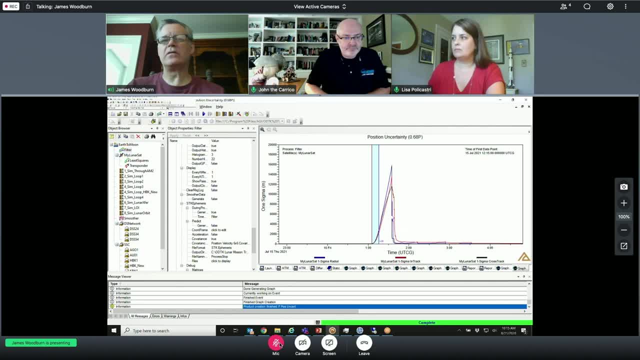 the uncertainty that the spacecraft goes through that maneuver, and this is only modeling: a one percent uncertainty in the thrust and one percent, i'm sorry, one degree uncertainty in the pointing direction of the maneuver. and yet you can still see how rapidly the uncertainty is growing because, as john you mentioned, this maneuver is big. this my particular scenario. this was a little over 800. 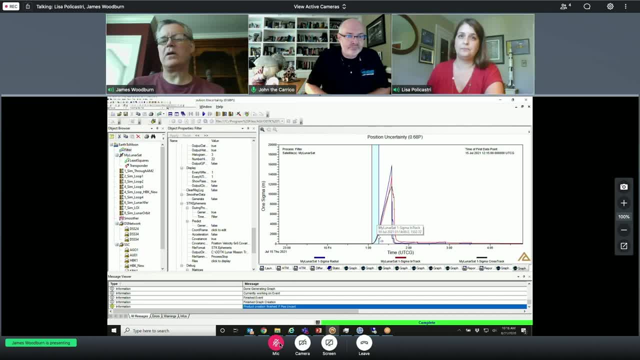 meters per second. you know just a one percent uncertainty in there and you're looking at eight meters per second of you know uncertainty in that maneuver and that grows very rapidly in terms of the orbital position error. so you know there is a need to get a contact very soon. 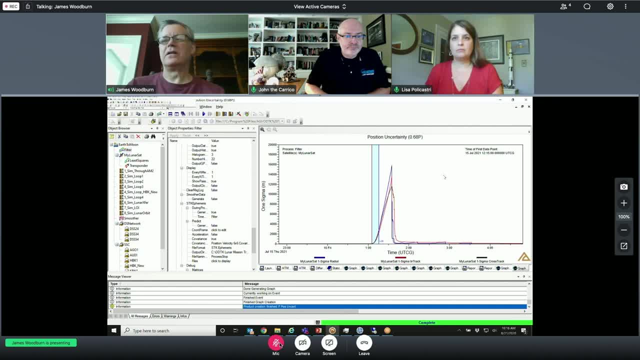 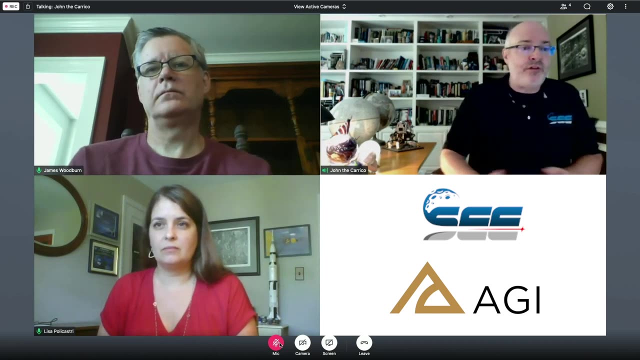 or as soon as possible after the lli maneuver, so that you can, you know, keep this error growth founded. and in fact, a lot of times this becomes a system engineering issue where the orbit determination somewhat innocently said: oh well, if you have a five percent uncertainty on your. 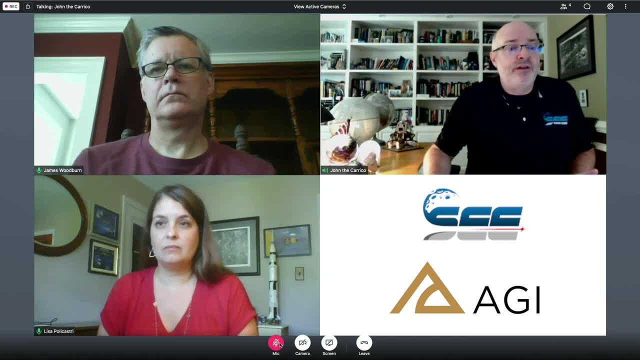 maneuver. you're going to have to do something about it, and then you can. from a system engineering point of view, you can either put a greater requirement on the propulsion system and say, well, you need to get the uncertainty down because we have this other mission goal, or we want to spend less money in the propulsion system. let it have a higher. 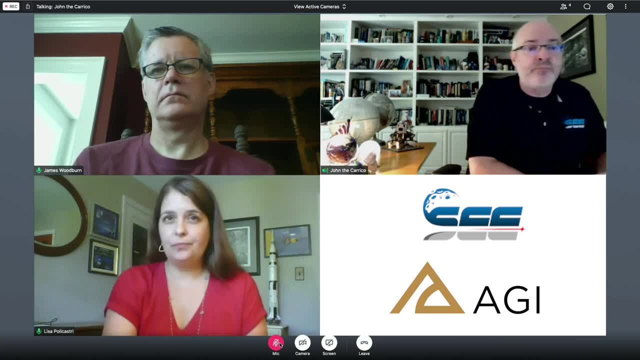 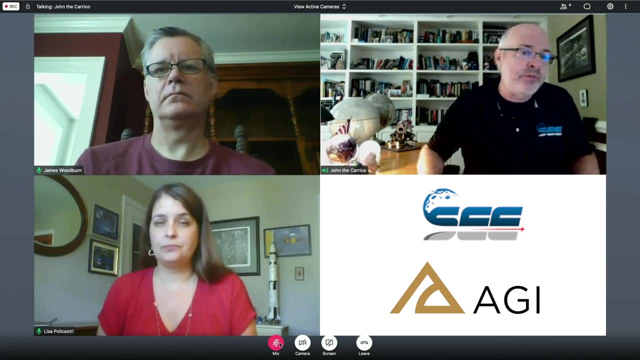 uncertainty because it's cheaper to buy tracking gases. so there's a whole system-wide optimization that i think. um, again, rodney danger has a lot to say about this, but i think it's a great way to think about this. but i think rodney danger field getting our respect. i think uh, a lot of times. 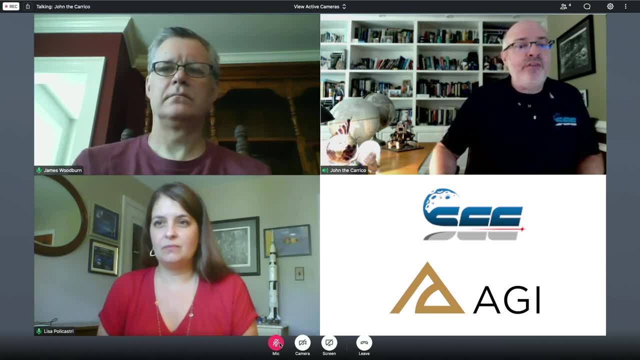 orbit determination is left out of that until the very last minute and they say, oh, you know, and they assume that orbit determination is, it is a done thing, which for geostationary satellites and for leo's- we've kind of been spoiled now, um, because it's, it's almost a commodity capability where 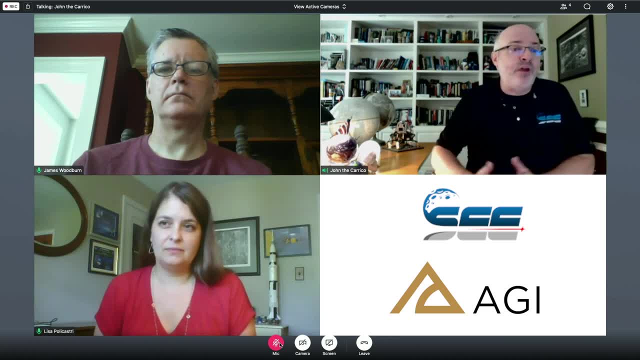 going to the moon you're very sensitive to. is your antenna even pointing in the right direction when you capture so you can get tracking data? if you know, just putting an omni-directional antenna on your spacecraft, um, like on the laddie mission when we were doing a capture at a low inclination? 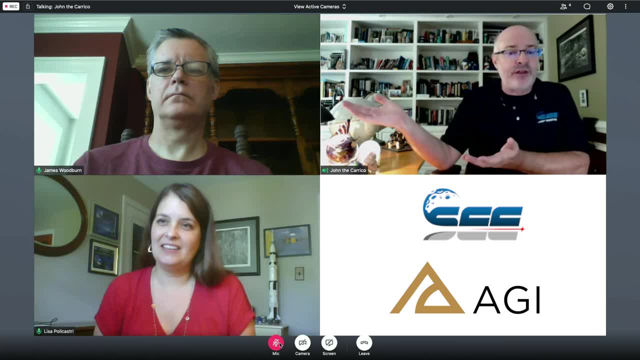 around the moon actually retrograde to very high inclination. during the maneuver we were from the earth. we were actually looking at the flames coming out of the satellite. so can you close the communications link during the maneuver? another way to do that is to put the antenna in the right. 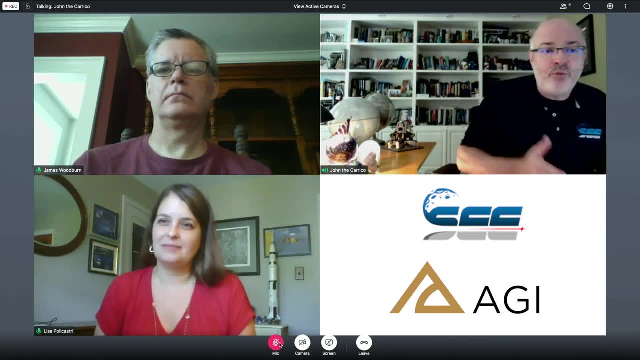 position and see if theCDC can be located in the right position and see what that means. you're going to have to wait for the spacecraft to get possible and you want the channel to be able to see this, or always have to wait for the spacecraft to get possible and this kind of thing. 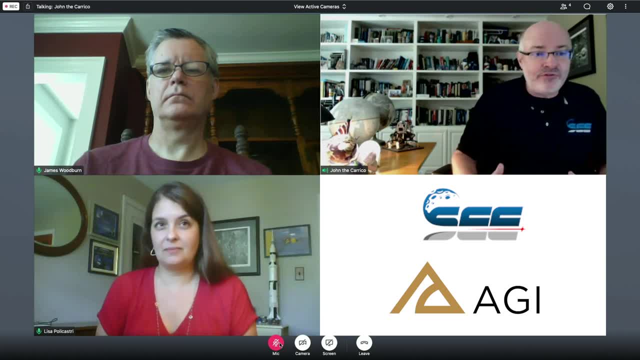 can be done if the idea is to just close the girth with the antenna. but the goal is to be able to be able to track a asset of a spacecraft. if it's possible and if you have to wait until the manoeuvre is done, and if not, do you have to wait till the maneuver is done- reorient the spacecraft and start. 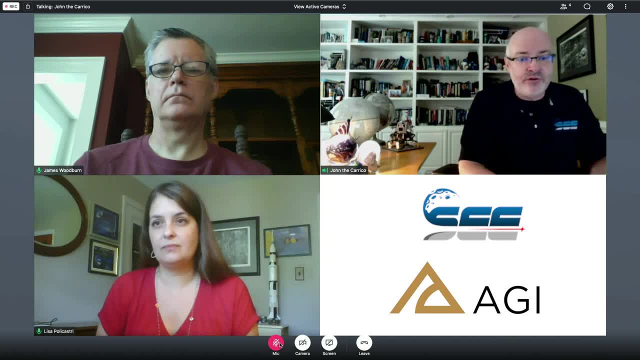 tracking right away. and You know, Lisa, you said you're going to change your maneuver plan based on orbit determination. Yeah, and I think some of these other considerations are: what is your mission going to be doing? Are you just going to- I should say, just going to land? 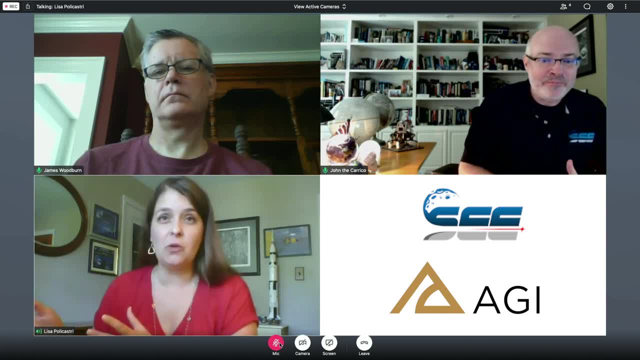 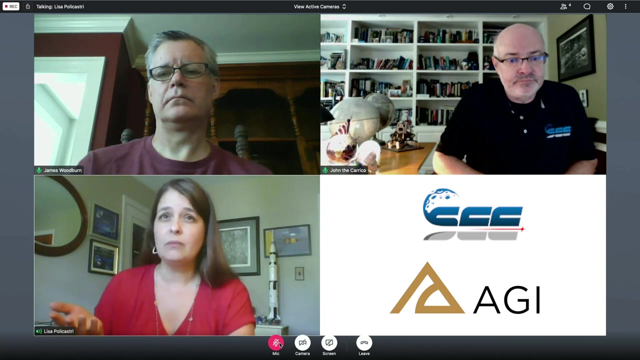 Are you going to land Or are you going to be in orbit for a while and do science or other types of observation? So that also comes into play with what OD air analysis you can do, For example. you know, if you're an orbiter you may be only able to track a certain amount of hours out of every day. 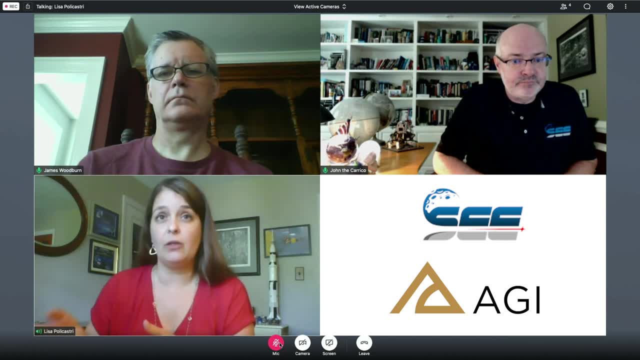 Because what John was talking about, the attitude, how the satellites orient. It may have to be oriented in such a way that you can't do communications to Earth if the measurements from the payloads have to, you know, drive the attitude of the spacecraft. 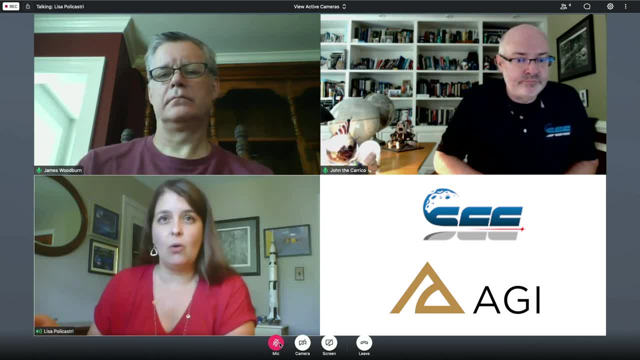 So we have to look at different tradeoffs, sometimes with the scientists, to say, okay, how much data do you need to collect per day to meet your mission? And what does that mean for communications attitude? Can we not talk? And what does that mean for the satellite from Earth during all of those times? 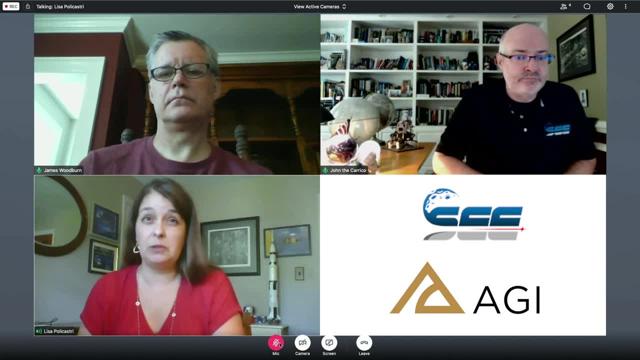 And so you may be really constrained or just actually sort of playing, trading off some things with the scientists early on to say, okay, well, in order for you to know where your satellite is going to be, to plan your science, we have to have so much tracking data in order for you to do that successfully. 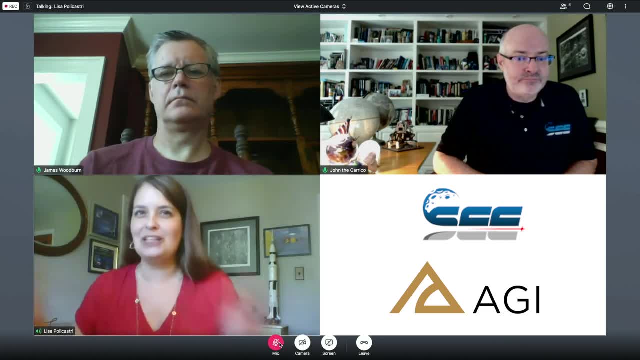 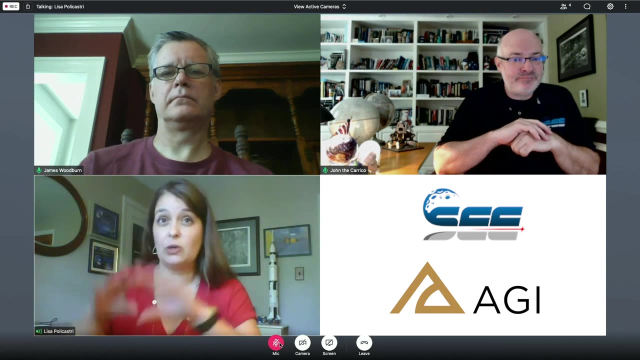 So maybe you can back off on that a little bit. Do you really need 23 out of 24 hours A day of science data? Probably not. You want that. You probably don't need it to include your mission. So you know you're playing some games like John, you brought like systems engineering sort of like from a whole system. 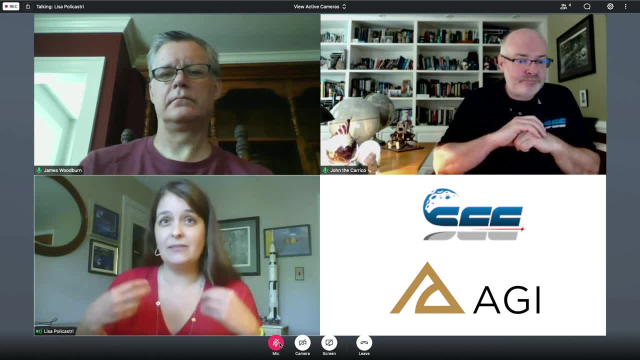 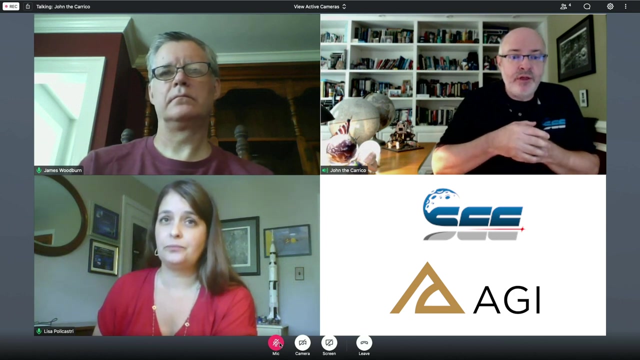 What do we want for tracking to be able to actually meet the science requirements, The science you know when you're looking at uncertainty in the orbit, when they're doing their science. Well, on LANDy we had some really tough to meet orbit prediction capabilities so they could point the science instrument. but I think we negotiated that we got what? three to five orbits after every maneuver just for tracking, so we could get back on, get back on track. 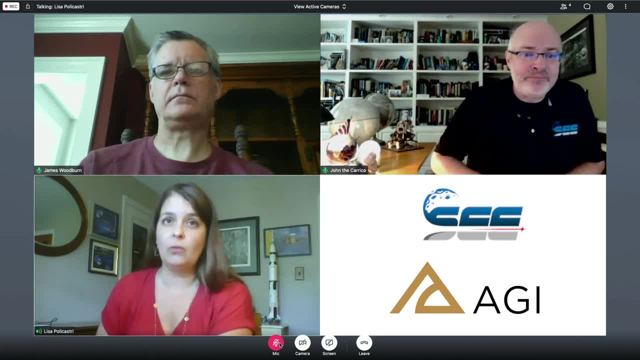 Yeah, there was definitely some negotiation with and we did a bunch of trade-offs using simulated tracking data, like you know, that ODTK let us do. Yeah, The other thing sometimes is when we're looking at tracking measurement type versus, like the spacecraft capability, you know, traditional ranging or sequential ranging from the DSN. that takes up some of your, some of your length budget. 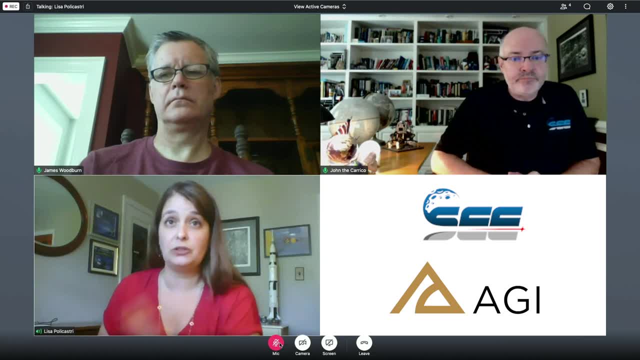 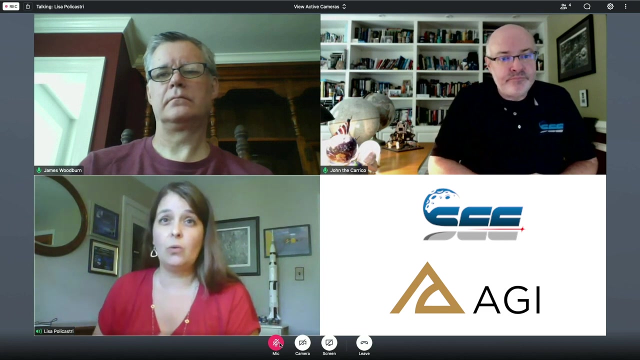 So your length margins are, you know, different whether you're doing Doppler or Doppler end ranging, And so we, We have to decide: okay, well, maybe we can live with Doppler only because during these communications passes they're also going to be downlinking science data or they're going to be, you know, doing other spacecraft activities, getting telemetry uploading, and so maybe we can't get ranging during those passes when there's other heavy activities going on during those comms passes. 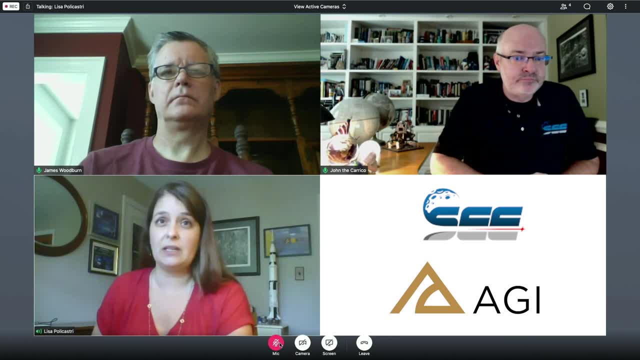 So we can do things like do some trade studies with simulated data, saying, okay, Doppler only is fine, We only want some ranging once in a while, And you know, maybe it's at night when all the other flight controllers are asleep or something, so they're not doing commanding. 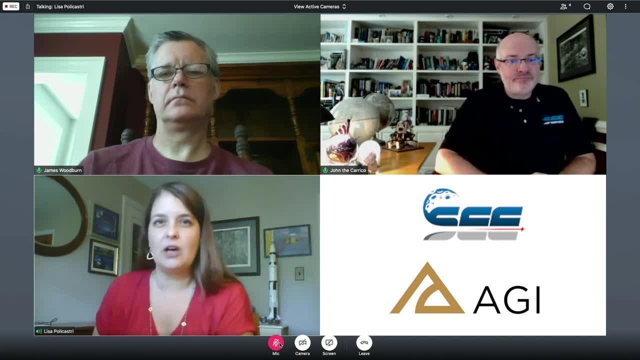 Yeah, You can play those games too, but still there's a lot of trade-offs to talk about. Some ground stations are now experimenting with the or doing the regenerative ranging, which uses less bandwidth, but it's not every ground station. 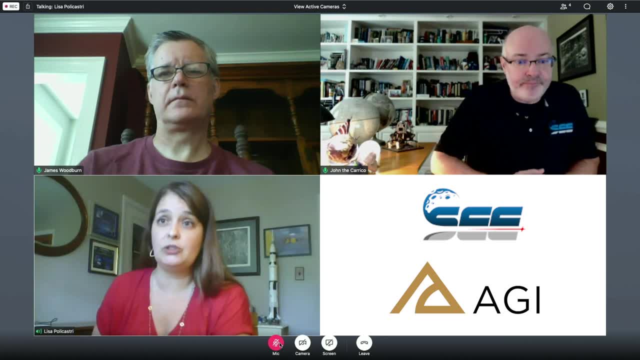 Not every ground station, not every transponder has the capability of doing It's using the regenerative pseudo-noise ranging Right. Might have said that out of order, but yeah, Yeah, all those words. It's being proposed on mission. 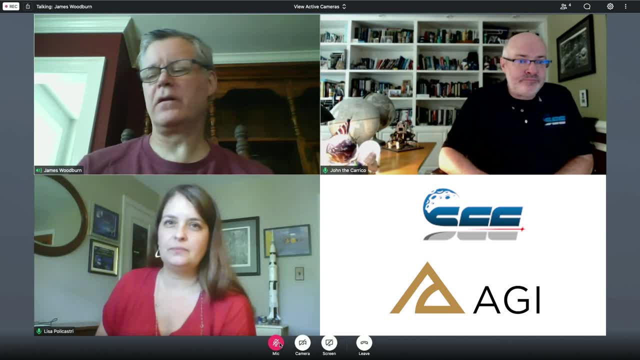 And there's another aspect to this whole trading back and forth right between science time and tracking time, And that has to do with the geometry of the tracking systems relative to the orbit about the moon. if you don't have a really heavy tracking schedule, then the orbit accuracy that you can get from your 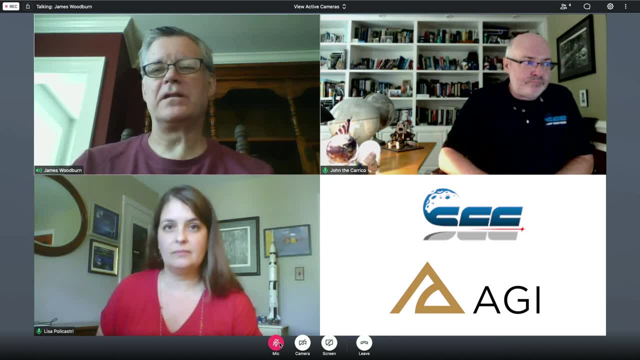 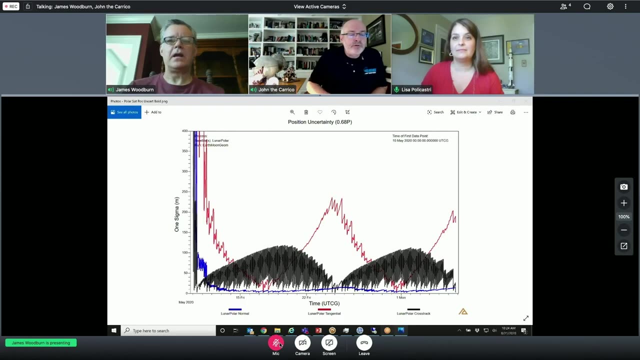 orbit determination process. it actually follows a cyclic pattern based on that, that geometry. so you can see this here. yeah, this is showing, uh, how the orbit uncertainty from the orbit determination system is varying over a month, and what you can see is that, while the red here is representing in-track uncertainty, and you can see how it has a cyclic 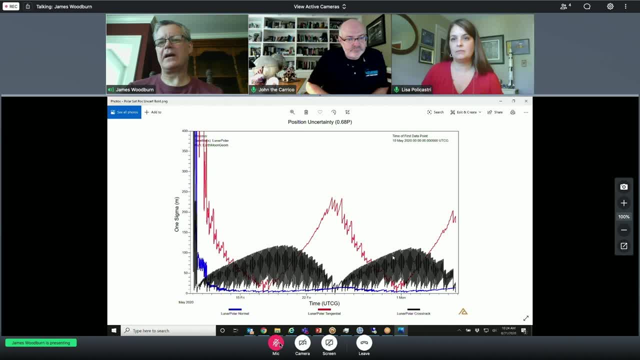 pattern to it. and then the black is measuring cross-track uncertainty and you can see how it also has a cyclic pattern. and what's going on here is: the fact is that the geometry of the orbit relative to the ground stations changes throughout the month, so the orbit is basically staying fixed in inertial. 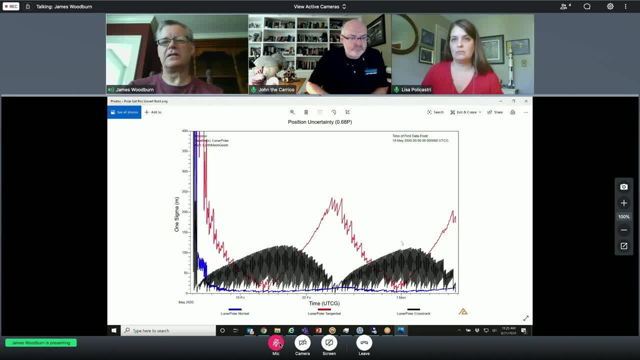 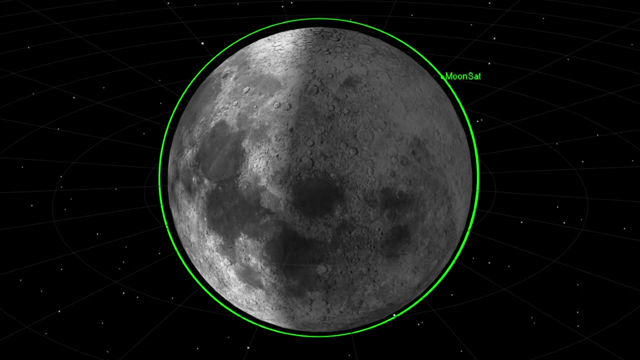 space as the moon goes around the earth, and so what you have is you have two times during the month when the ground stations are almost in the plane of the orbit, and then two times during the month when the ground stations or the line of sight from the ground stations is basically perpendicular to the orbit. 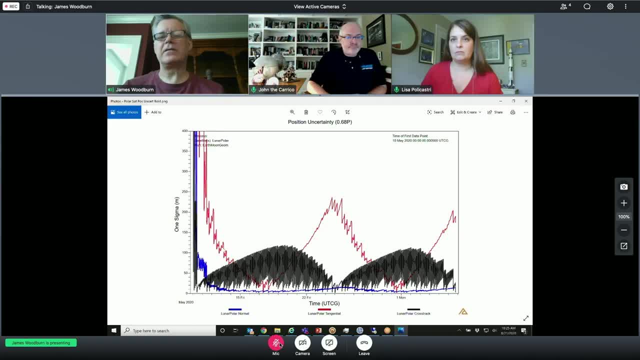 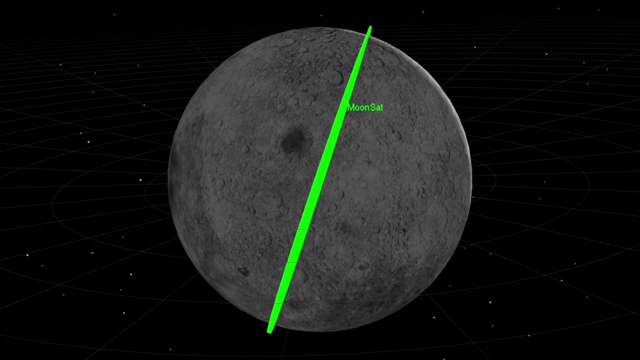 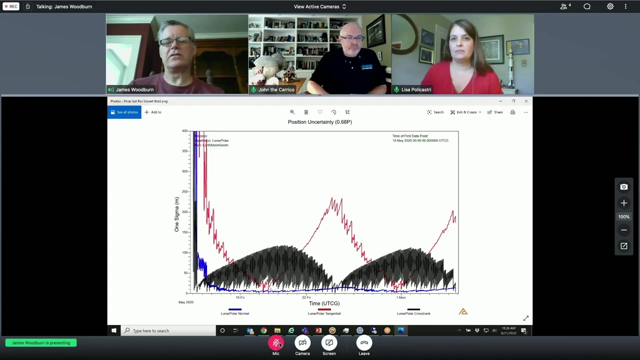 and so that affects the type of orbit accuracy that you can get. these low points in the black uncertainty correspond to when the ground station is inside, basically the orbit plane, because you're looking directly at the spacecraft either coming towards you or going away from you, and that gives you really good accuracy in 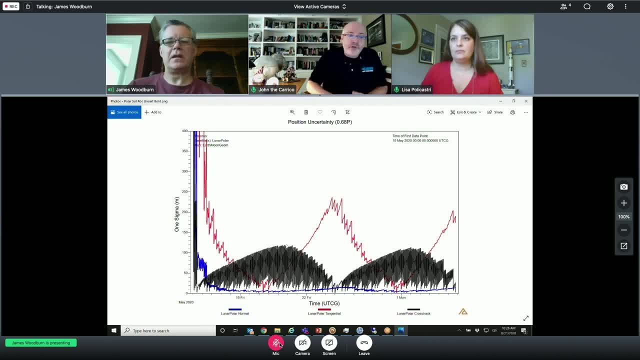 the in-track direction. but at the same time- and that's Jim- when using a Doppler measurement, this is range and Doppler yeah, because they're both line-of-sight measurements, they're both measuring just purely along the line between the spacecraft and the ground station. because 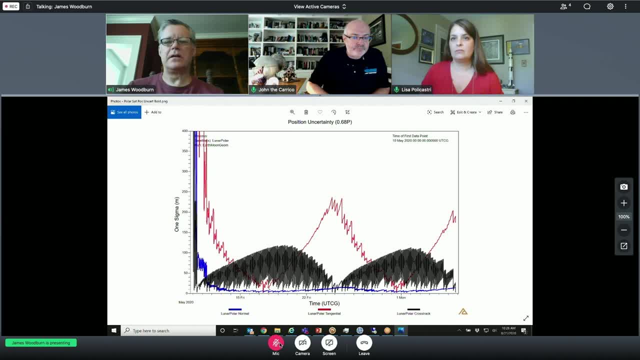 angle. measurements at the lunar distance don't really help us much to give us, like in a low Earth scenario. right, you have azimuth and elevation complementary to the range of Doppler, providing measurement information in different directions. but those measurements become so weak at lunar distance that they don't really help. and then when the spacecraft- I'm sorry when the 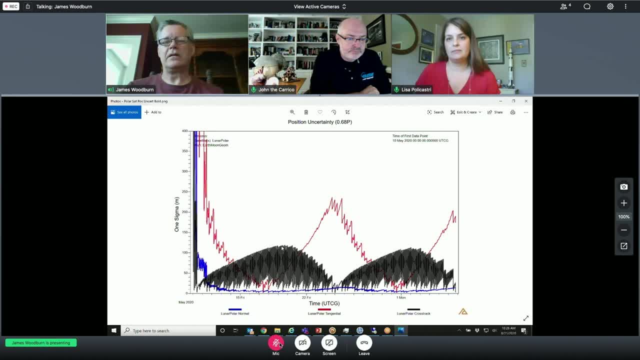 ground station is in the in the orbit plane as well, the sensitivity to the cross track error becomes much less, and that's why you see the cross track errors go way up during periods when the in-track error is low and you have a corresponding thing going on when you're looking. 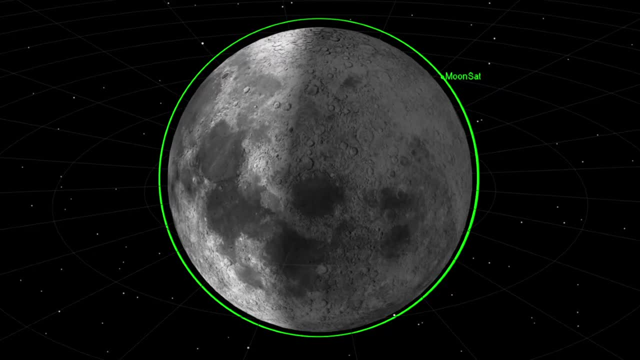 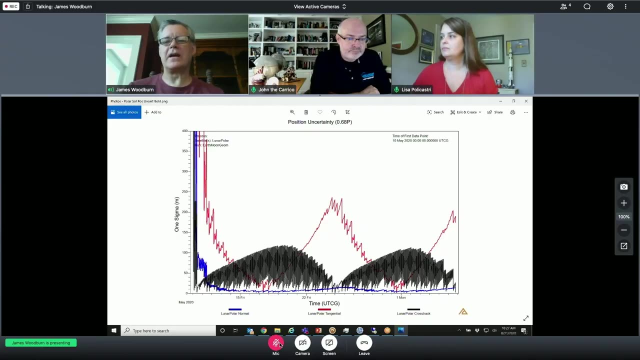 at the orbit plane from a perpendicular direction, the cross track uncertainty goes way down, because now that's exactly what we're measuring- measuring directly in the cross track direction. but the in-track uncertainty goes up because we're much less sensitive to the in-track errors under that. 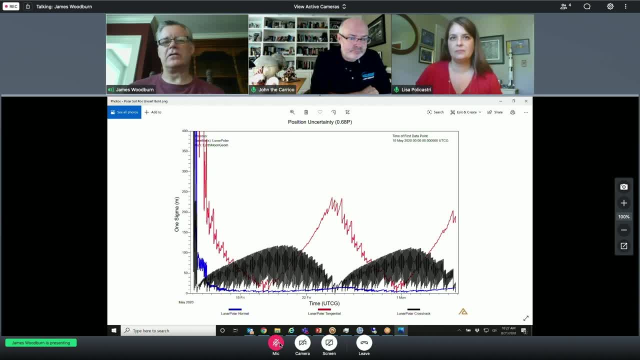 geometry. so when you're, when you're trading back and forth between tracking time and science time, and all depending on what type of accuracy your science requires, you may need more tracking at certain times of the month than other times of the month- meet the science requirements because of the geometry is occurring between the. 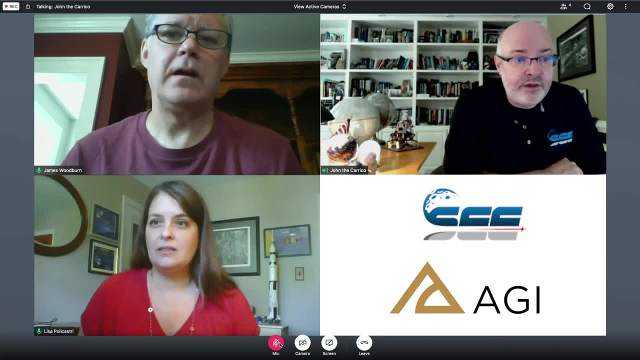 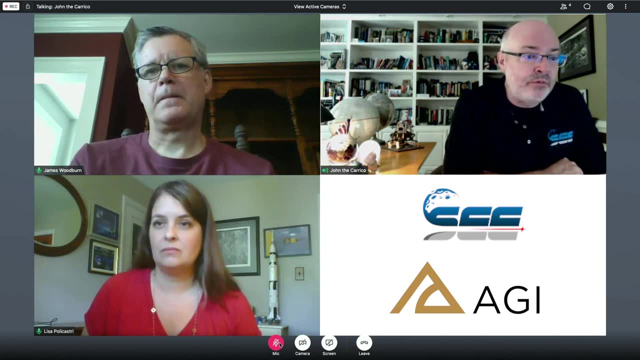 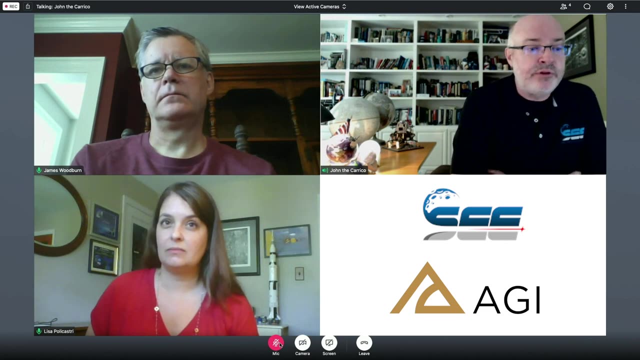 ground stations and, just to say it, if you're not on the science mission and you're on a landing mission, you still care about predicted uncertainty. because when you go to do your final maneuver to land, usually what you do is you take the uncertainty that's calculated by the orbit determination system and you use 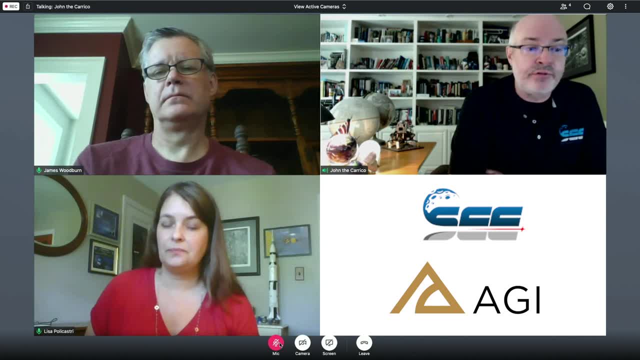 that as your initial starting point for the onboard guidance for the lander. so you're still managing uncertainty in managing that schedule and making sure that you do or don't have line of sight, depending on what. what are the more important terms for the onboard guidance systems? you know what does it need for. 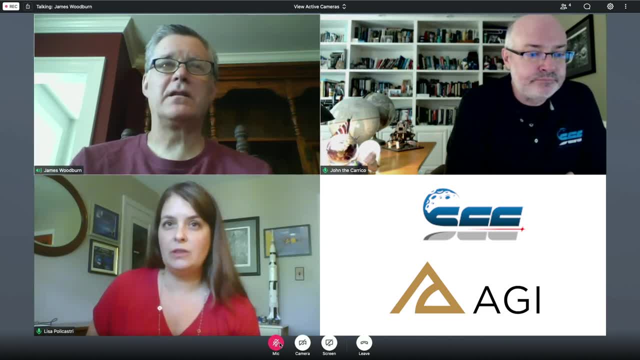 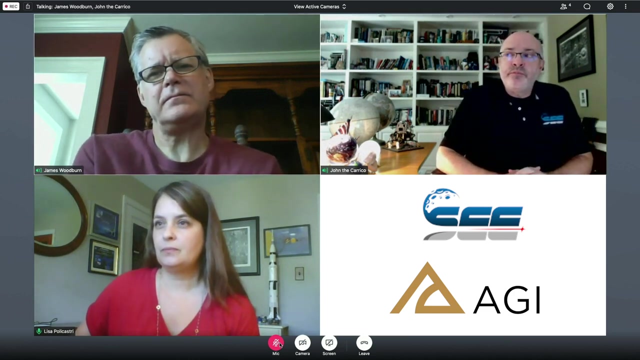 its initialization. now, how long, john, like on bear sheet, how long prior to the beginning of the final, final descent, were we able to affect the orbit based on, you know, ground-based orbit determination? what was the cutoff? what was the cutoff? i forget what the cutoff was. was it on the order of a day? 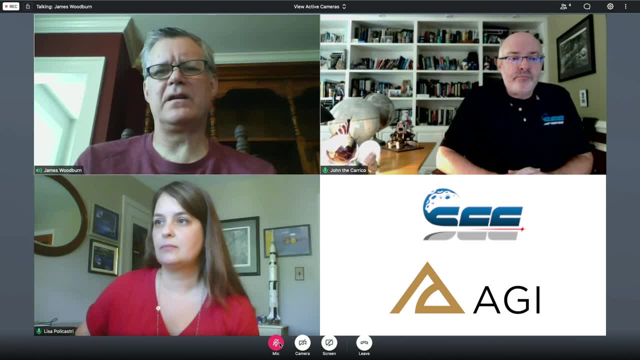 it was a significant period of time, i think. yeah, for the last update. yeah, i think we put that in our paper but i don't remember it off the top of my head because that kind of goes into your discussion of, like you need to use that orbit uncertainty. 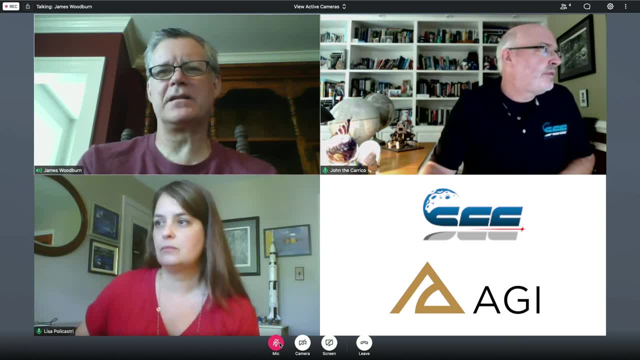 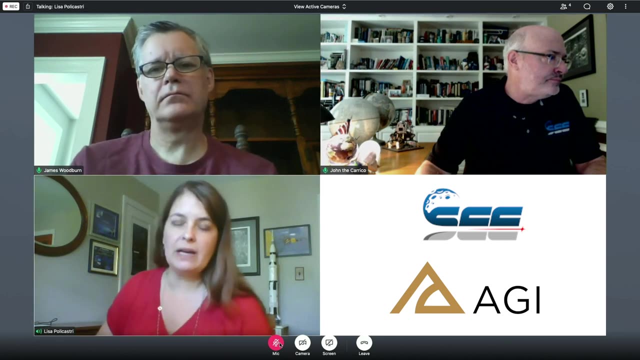 from the od system to kind of feed the landing process, but you're not getting benefit of tracking data right up to the point. let me write the procedure. just go back to the graphs you were showing just now. that was for an, uh, what i would call a polar. 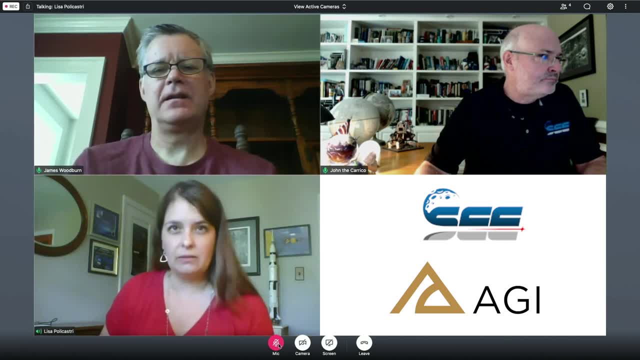 lunar orbit, right, right, and so like, for example, lro is in an orbit like that that you showed. yeah, where, uh, you know other missions that are just for equatorial orbiters be different patterns, but a lot, of, a lot of these. you know upcoming missions or proposed missions, you know people. 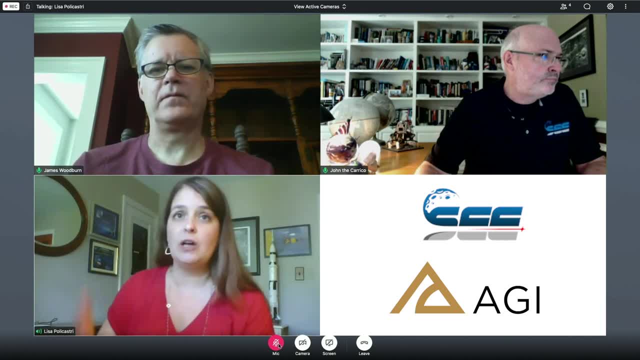 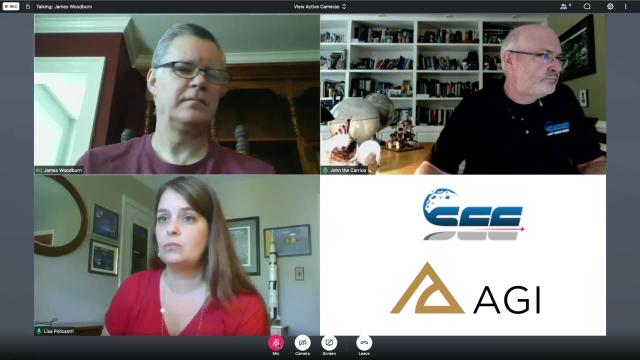 are interested in doing polar um, they want to, you know, observe the poles and look at the ice um land at the pole. so a lot of the you know there's a lot of interest in getting into the polar lunar orbits that you were just showing. yeah, any mission that's going to want to have full ground coverage. 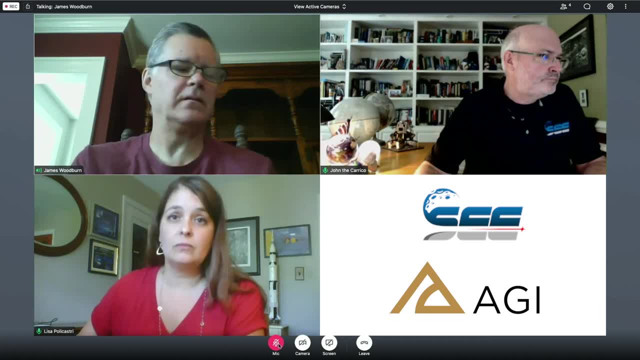 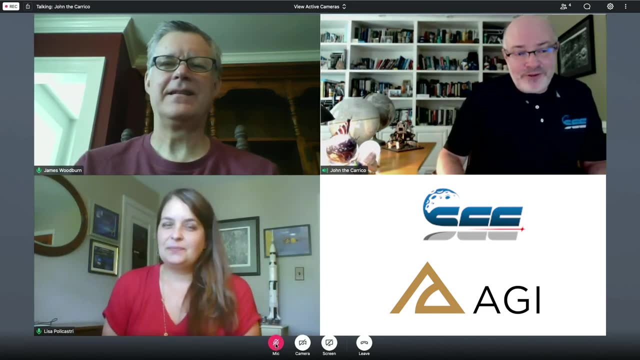 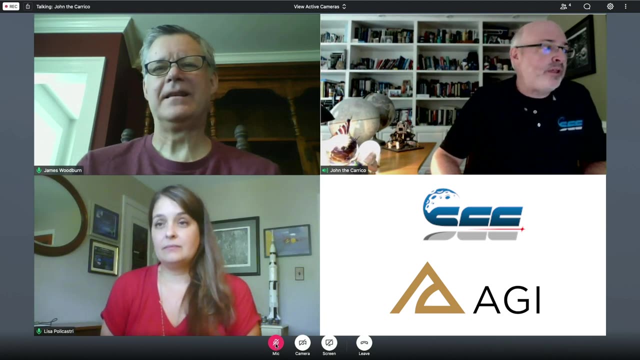 probably going to be in at least a high inclination orbit, if not polar. so, um, so, jim i, i uh looked it up through the magic of video editing. i looked up the timeline of maneuvers: um, for the bear sheet mission And it was pretty sporty. We captured around the moon with a lunar orbit insertion. one maneuver on April 4th. 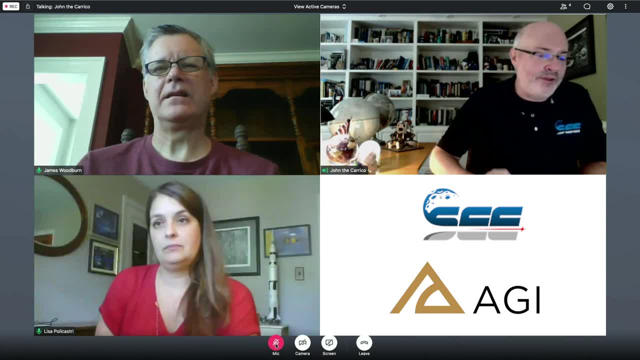 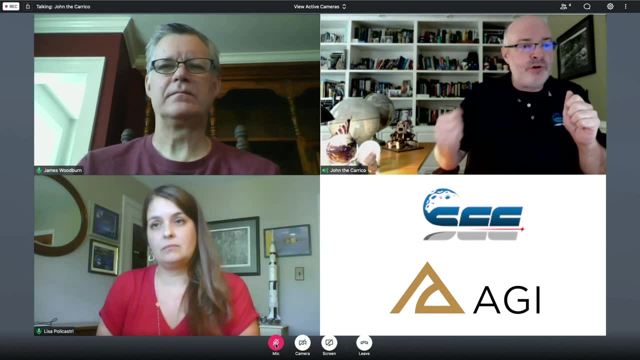 Then we did a maneuver on the 7th, the 8th, the 9th and then the final maneuver. So we're kind of like in a circular orbit. We do a final maneuver to lower Paris lean to about 15 kilometers. That took place on the 10th And then I think we did about 15 or 16 revs there And then they started landing. So from the final, from the final maneuver to the initiation of the land was, I think, only 15 or 16 orbits. 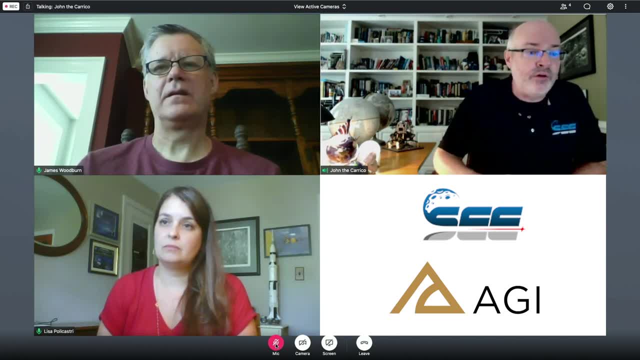 That's challenging to get the orbit determination, you know, and then the predicts to see it on board. Yeah well, that's, that's especially important. It's really scary thinking about that. Paris lean altitude- What did you say? that was 16 kilometers. 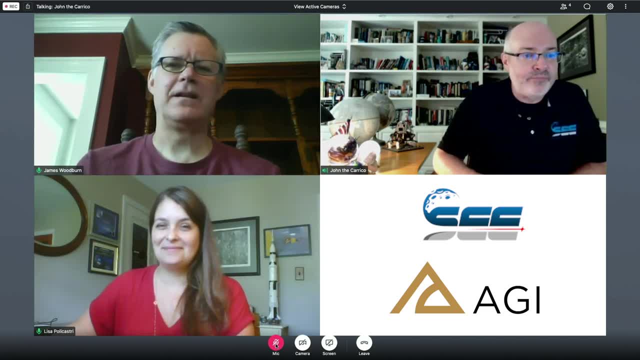 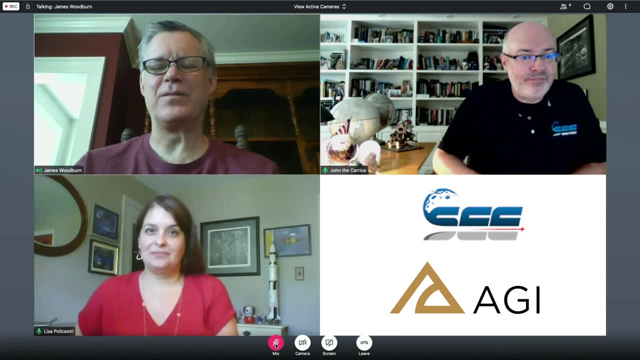 Yeah, somewhere around 15 or 16 kilometers, if I remember right. Yeah, So that's another big difference between what you can do at the moon and what you can do at the Earth. right, There's no way that you're going to be flying a satellite at 15 kilometers altitude around the Earth. 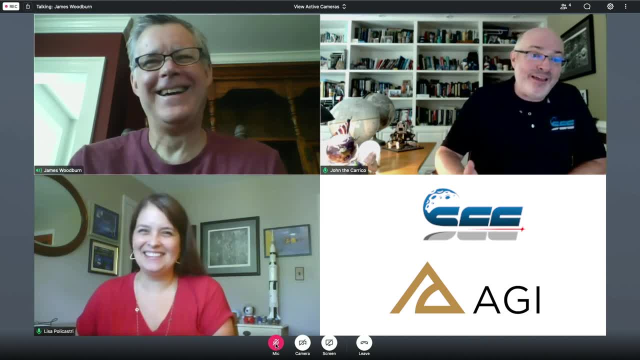 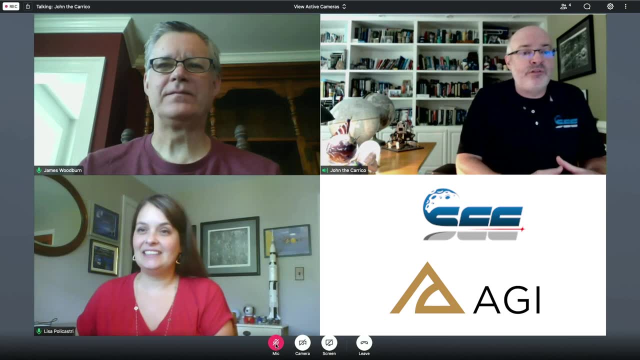 Well, you're not going to fly it very long. Well, on LADEE, the scientists asked us to, in the extended mission, to go at 15 kilometers altitude. So we actually brought terrain into Satellite Toolkit and we're plotting the OD uncertainty ellipsoid with respect to terrain. 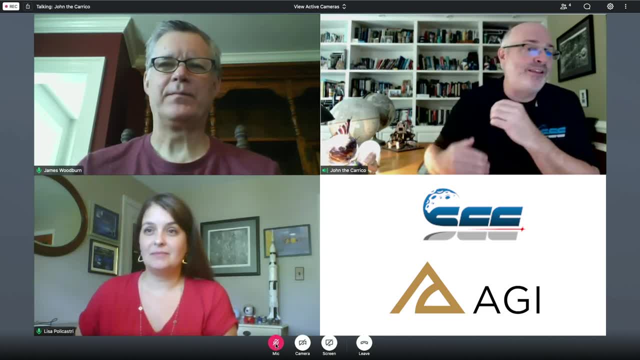 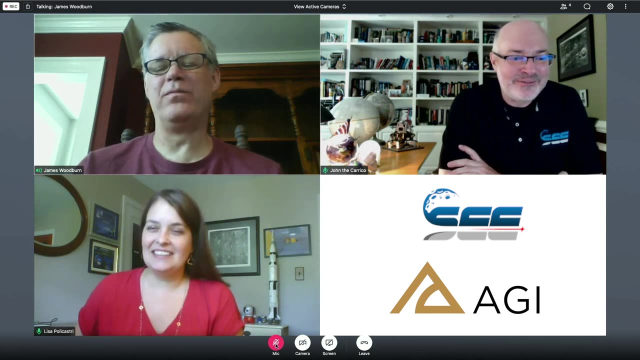 And there were times when if we had got like a four sigma uncertainty, that was scraping the dirt on the moon. I'm sorry we're supposed to use the word regular, right? Of course that flying that low brings other types of requirements. We're used to being around the Earth and flying with a 50 by 50 or 70 by 70 gravity field, And that's just not going to cut it for these kind of operations at the moon. when you're down that low, You could be looking at 150 by 150, 200 by 200, or even larger gravity fields. 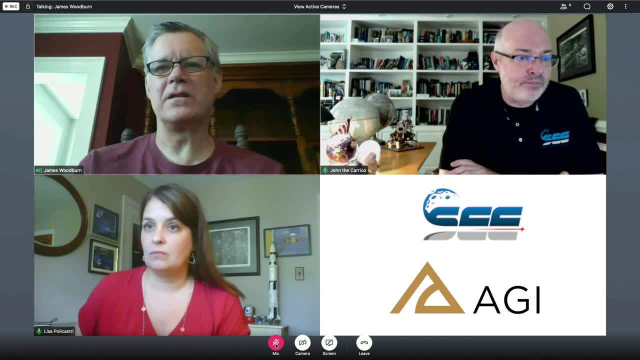 Oh, yeah, for sure. And now we're looking at 150 by 150, 200 by 200. Yeah, for sure. And now that GRAIL has the gravity models out there, the uncertainties on the gravity field have gotten a lot smaller. Right, Actually, my first mission that was a lunar mission was Clementine. When we started that, I think, we had a 16 by 8 dozen Ferrari gravity model or something. Huge uncertainties in the gravity, So we designed the orbit to be really high. 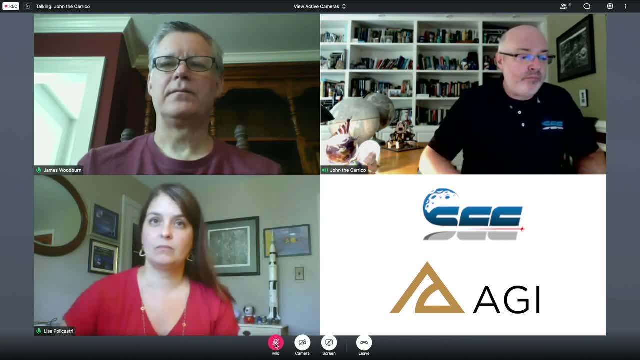 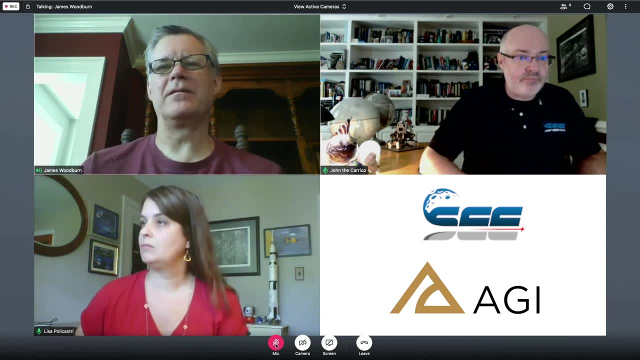 The GRAIL gravity models totally changed where the problems in lunar prediction are. It went from being 100% in the gravity field to now solar pressure can be your largest source of dynamic model uncertainty. Yeah Well, one of the problems we had on the Clementine mission. The Deep Space Program science experiment, which was a NRL NASA mission when I was at NASA, Goddard was. it was the first mission that Goddard had done around the moon in a long time, if ever, And so just configuring the software. 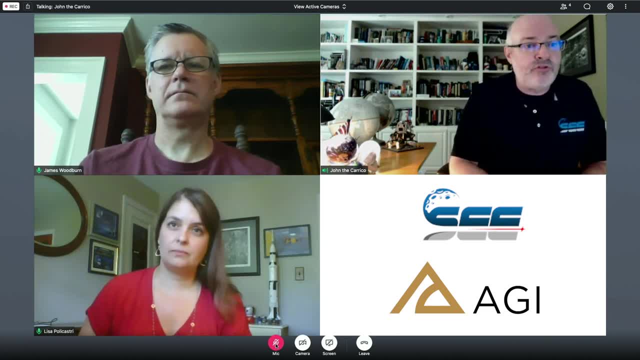 And we were using some mainframe based orbit determination at the time And there was an error there. But they had configured the software ahead of time to make sure that there was no atmospheric drag. There was no atmospheric drag on at the moon. They took all the input cards that had anything to do with atmospheric drag out. 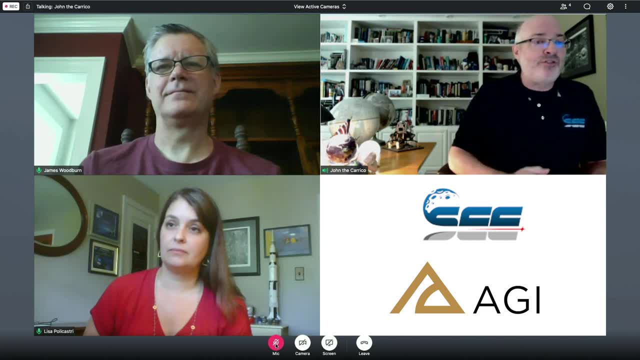 If I remember right, the software is written such that if there are no input cards for atmospheric drag, then it threw Harris-Priester on by default. So they're actually modeling atmospheric drag at the moon And I don't know if you guys have ever heard this, but have you heard about the restaurant on the moon? 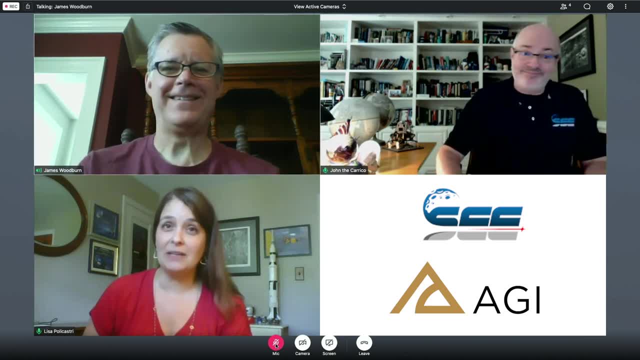 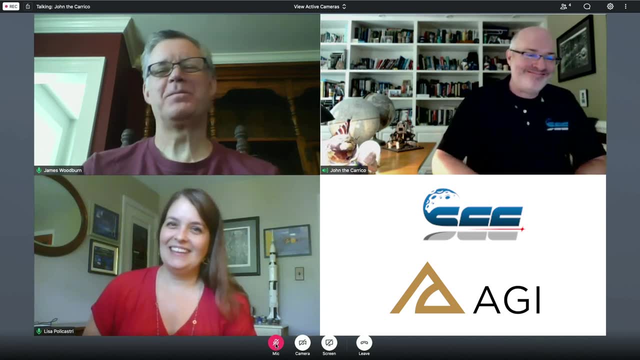 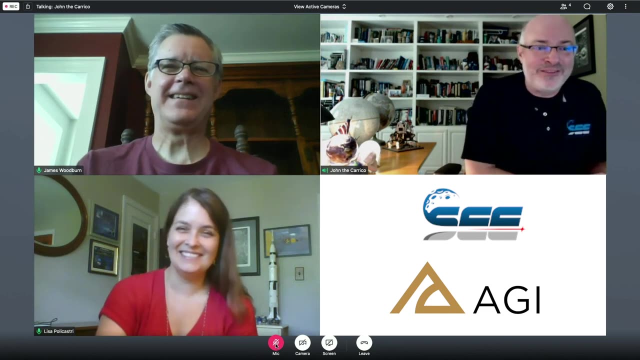 No, I haven't. No, John, Tell me about it, Believe it or not. there's a restaurant on the moon. It's got great food, but there's no ants. In any case, that is one thing that you think you don't have to worry about modeling around the moon, but make sure you don't model it around the moon. 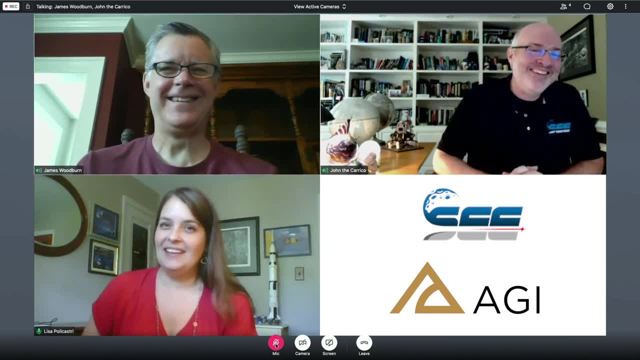 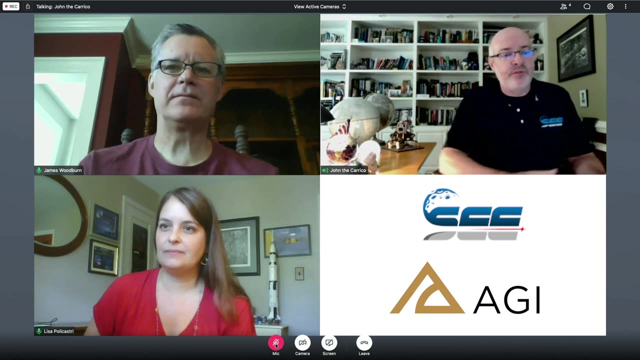 Right, Turn it off. But so solar pressure? And then, Jim, just thinking about it, when you fly over to sub solar point you've got an albedo. now, You know, from a thermal point of view, the thermal guys always say there's two moons, two suns. you know, on either side. 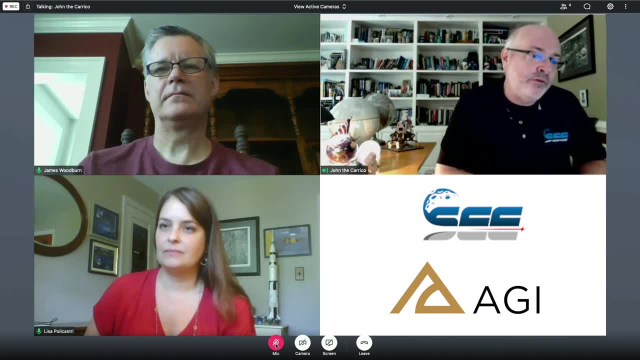 But I imagine if the gravity is well known now I wonder if you could start to seeing some of that albedo reflection, Especially at those low altitudes. Yeah, We only had a way to model it ahead of time to see what the sensitivity to the different courses were.